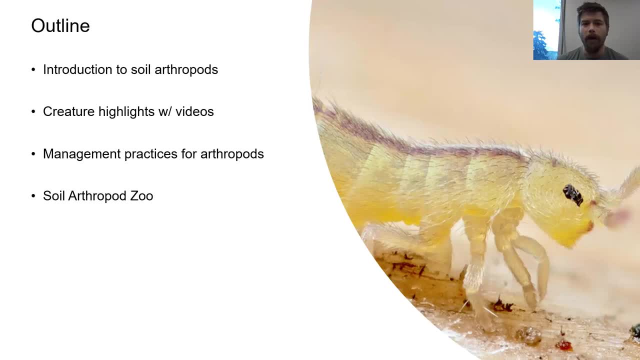 to start with an introduction to the soil arthropod fauna, And then most of what we're going to do is just take a look at some creature highlights, highlighting this fascinating group of organisms. I've got some great videos to share with you all, And then we'll round. 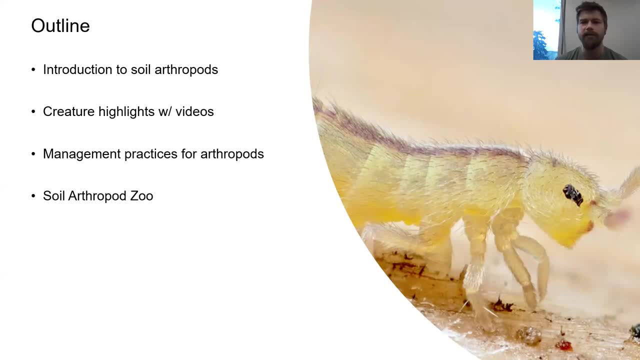 things out, talking a little bit about some of my PhD research focusing on looking at different agricultural management practices that promote these soil arthropod communities in ag systems. You see this soil arthropod zoo on here. Unfortunately, we're not going to be able to get to that today. 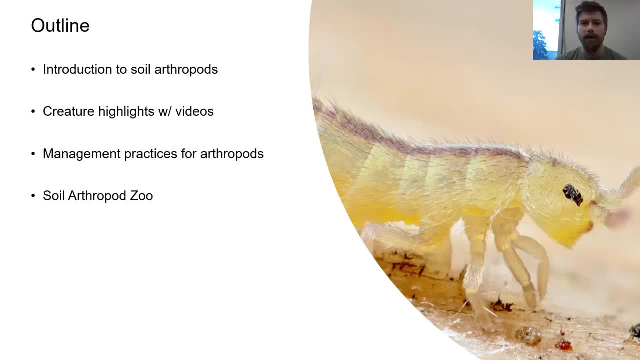 I actually do keep live colonies of these soil arthropods here at our laboratory And I was hoping to be able to share some of those with you with a microscope camera, but I'm not able to get that to talk to my computer, So we'll just have to spend some more time, maybe, with some questions. All right, So we'll. 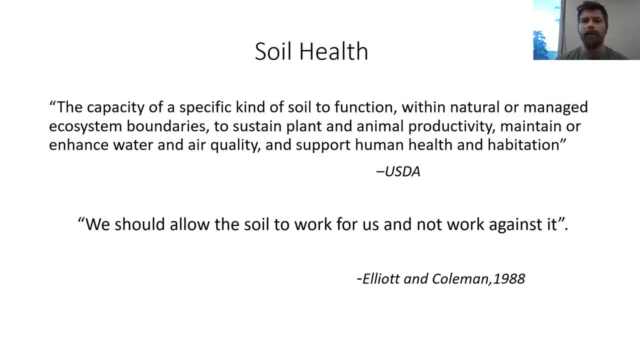 get going here. So I've got soil health in the title of the presentation- And this is a pretty popular, somewhat loaded term that we're hearing a lot about today- And I've got a couple different definitions on the screen here. This first one is from the USDA and it's a pretty long. 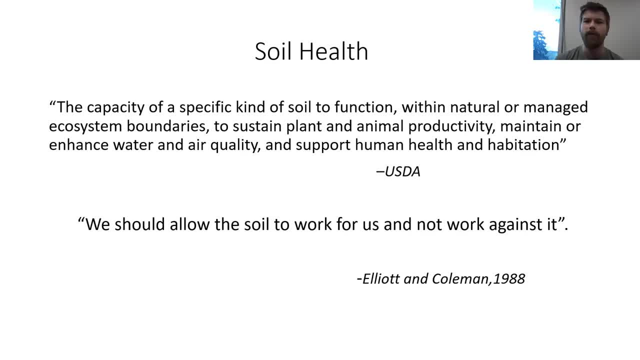 wordy definition, I won't read through it. I want to rather focus on the second definition of soil health that we've got here on the screen, which is, you know, we should allow the soil to work for us and not work against us. This seems like a pretty simple definition. 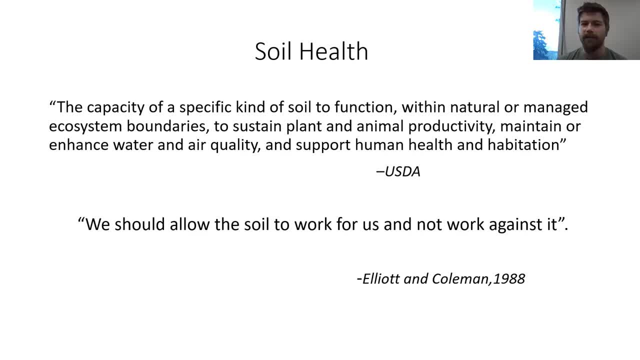 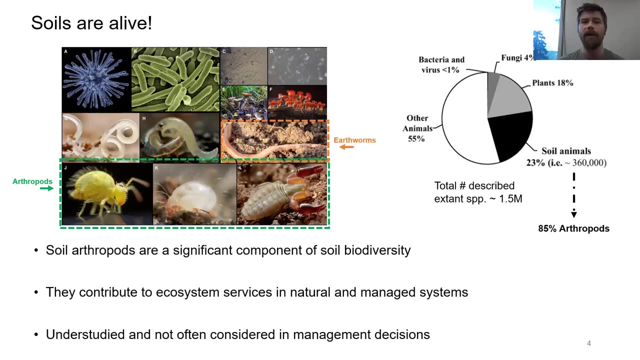 And I'm hoping that by the end of this presentation I've convinced you that soil arthropods are a critical part of what helps the soil work for us All. right, So jumping in right away. So soils are alive, As many of you all. 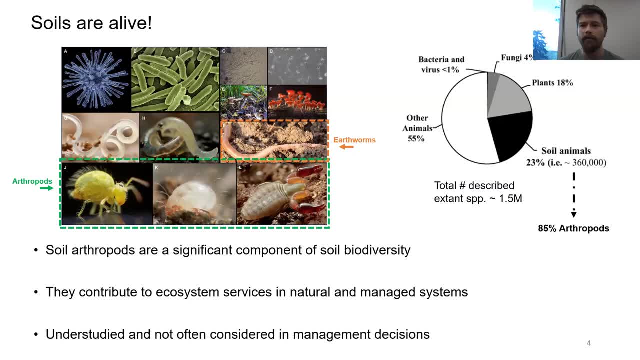 know. they are home to every kingdom of life on the planet, ranging from viruses, bacteria, fungi, all the way up to some of the larger mammals right, Like maybe voles and moles, things like that. You don't see those pictured here on the screen today: Soil arthropods. 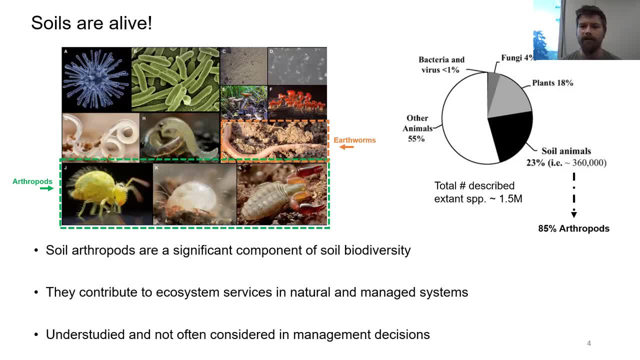 are a really large component of soil biodiversity. So there's about 1.5 million species that have been described, And of those described species, 23% of them spend all or some of their life in the soil And of that 23%, 85% of those. 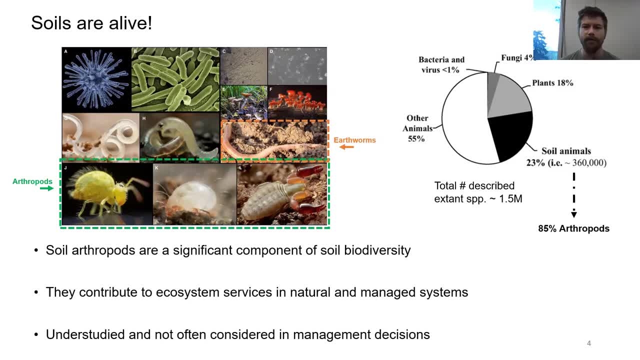 are arthropods, And so they're this really large, diverse group, and they're very important in contributing to ecosystem services in natural and managed systems. However, compared to some of their other counterparts that live in the soil, like earthworms and microbial, 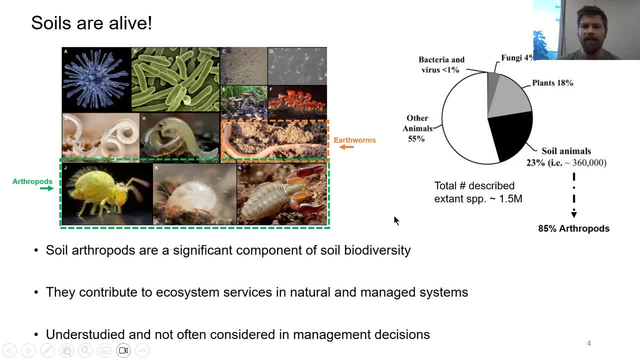 communities, as well as nematodes, to a certain extent. they don't really get as much attention And it's a relatively understudied group And I think this is a big gap in our knowledge. is what we know about soil, arthropods And 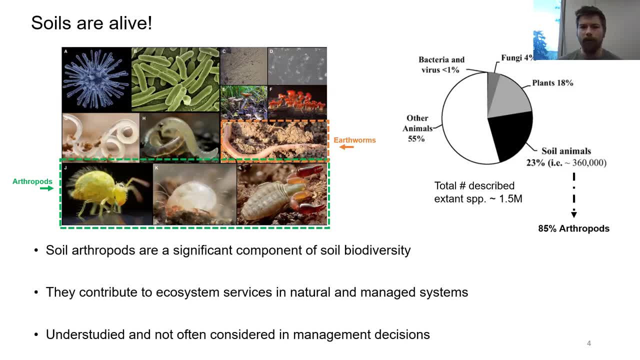 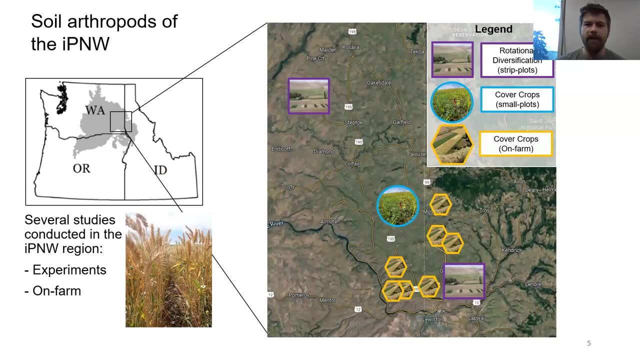 so I think it's a really important group to study and learn more about, And that basically has been the focus of my PhD research here at the University of Idaho for the last four years. So we're going to talk about soil arthropods today, of course, And a lot of the data as 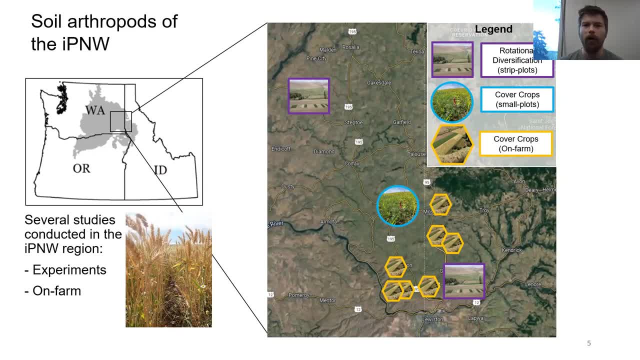 well as the pictures of the critters that I'm going to share with you, were all collected from agricultural systems in our region, So here we just see a map highlighting some of our sampling sites where we've conducted various experiments, or, in some cases, actually. on-farm studies Just to illustrate that we've done a fair amount of sampling And it's a great opportunity to get quite a bit of the information that we're getting from the sites. So let's go ahead and look at some of our samples. 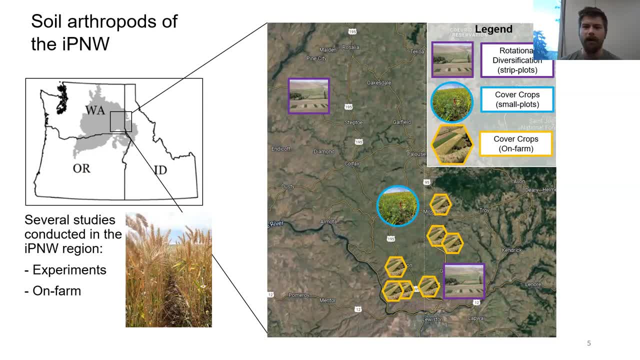 So here we have a map highlighting some of our sampling sites where we've conducted various experiments or, in some cases, actually on-farm studies, Just to illustrate that we've done a fair amount of sampling- sampling in this region in multiple different locations. 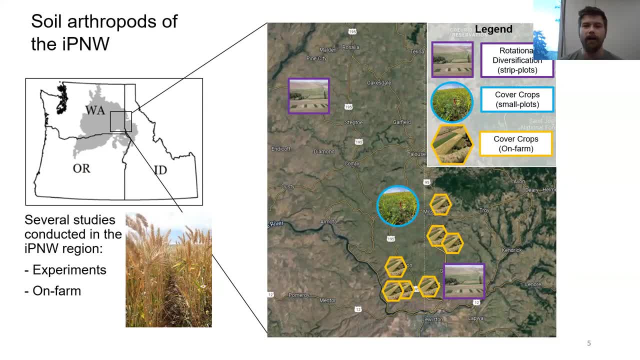 And this is actually kind of the. it is the first ever kind of look at these communities, the first ever sampling effort that's been undertaken to try to learn more about soil, arthropods and agricultural systems. So it's a nice set of data set. 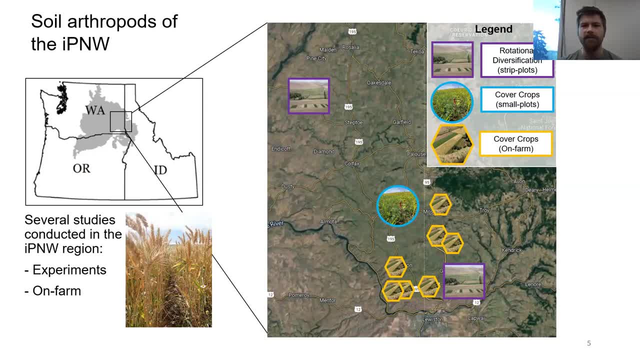 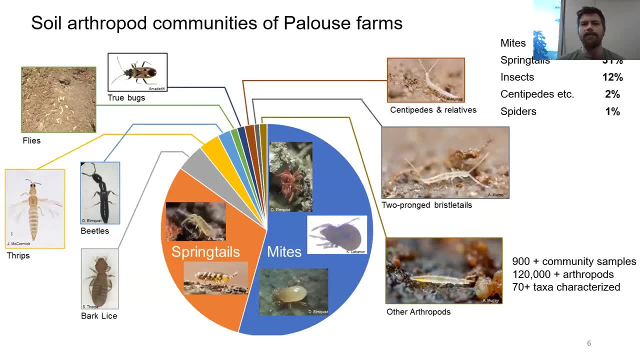 that's gonna hopefully serve as a baseline for monitoring changes in these communities over time. All right, so diving right into it. So this pie graph here is basically showing a rough outline of what the soil arthropod communities of Palouse Farms are like. 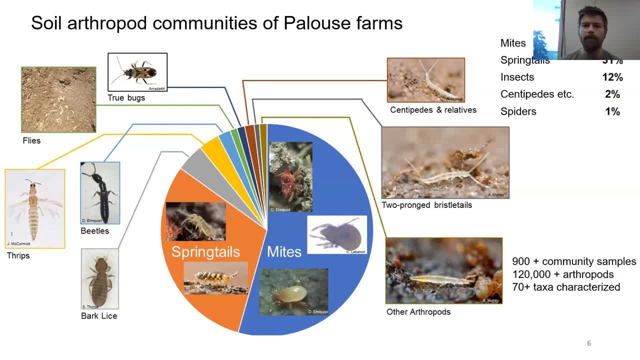 These are again based off of all of our sampling that you saw from those sites on the previous slide, And this includes over 900 community samples, 120,000 plus arthropods counted and over 70,000, 20 different taxa identified. 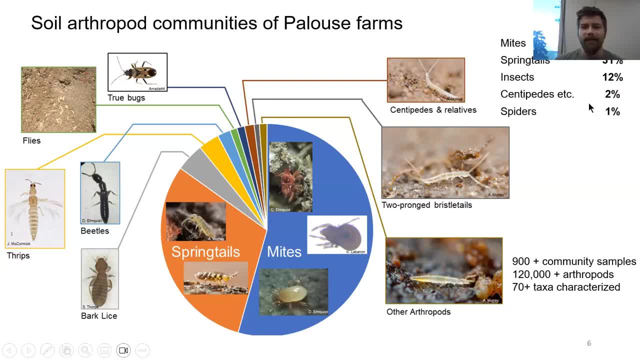 That's a very nice visual you have there, Yeah, thank you, And it's a really big data set too, So it's a really good again data that serves as a baseline for monitoring changes in these communities over time And, like many most soil arthropod communities, 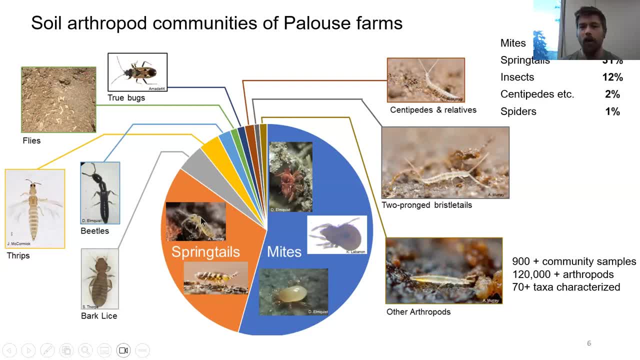 our soil. arthropod communities are dominated by springtails, also called columbula and mites, And we'll talk a little bit more about these guys as we move through the presentation. But they make up about 80, 85% of the arthropods. 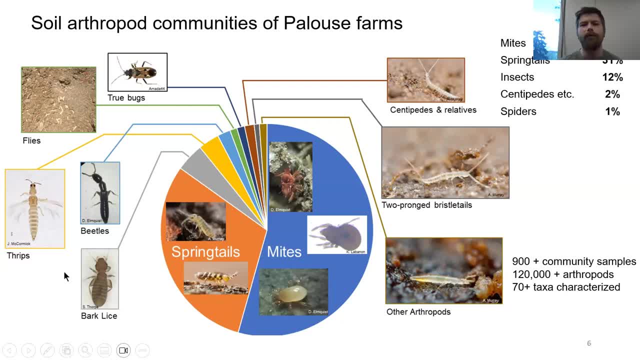 that we sampled so far. Other really important insects or prevalent insects that we sampled from agricultural systems include bark lice, and these guys are decomposers. They're living in leaf litter on the surface of the soil, breaking down, comminuting litter. 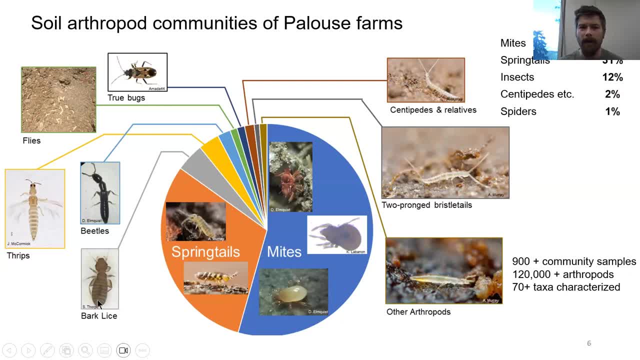 increasing that surface area which helps microbes come in and improve the quality of litter for nutrient cycle. Thrips were another big kind of surprising soil arthropod. We don't always think of them as soil arthropods. We'll talk about that a little bit. 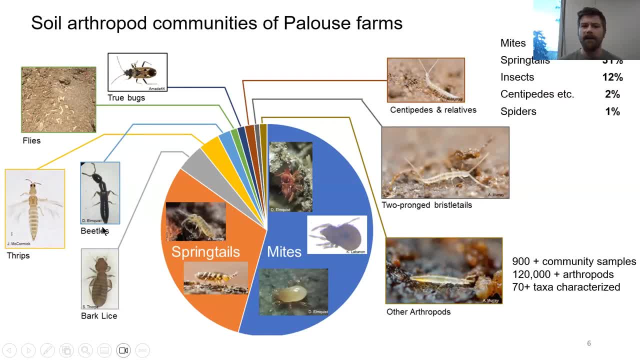 Beetles were another really prevalent group, And beetles are important because they include many different functional groups like predators as well as decomposers. And beetles were the third most abundant insect that we were able to collect from our communities. So that's what arthropods are. 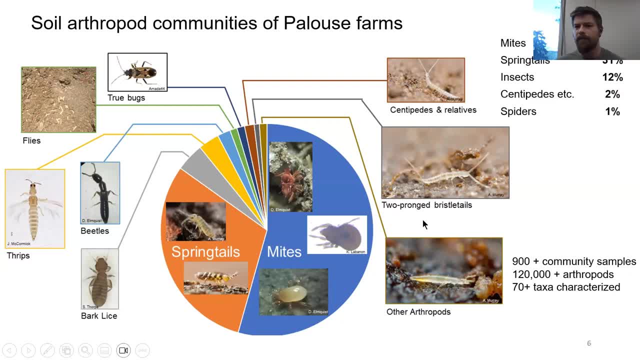 They're basically the most abundant insect you can find in the soil and they've been well known in the community sampling. Some other soil arthropods that maybe are a little bit less familiar to folks out there include two-pronged bristle tails. 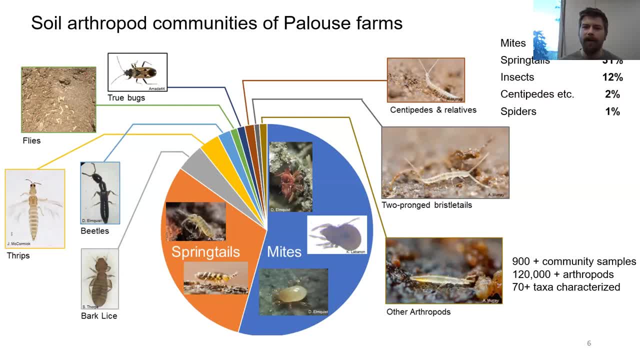 These are small, fast-moving arthropods that live in the soil, act as decomposers and predators. So again, they're providing a lot of different functions in the soil. And then there also are these- the name is the coneheads. 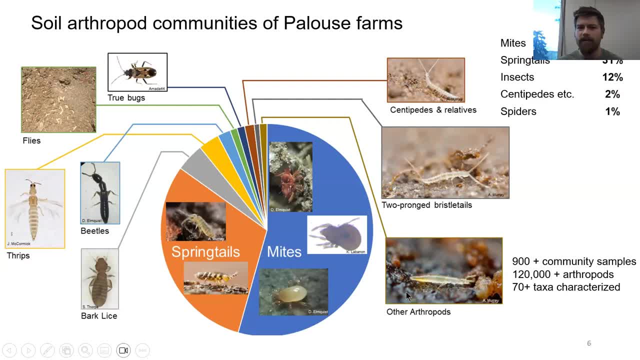 These were not extremely common in our samples, but again, I just wanted to highlight them here because they are a soil arthropod and they may not be familiar to a lot of folks. So, again, this is a large data set that we've collected. 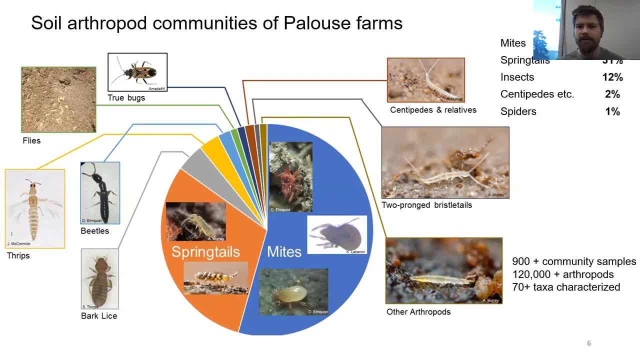 and hopefully it can serve as a good baseline for monitoring changes in these communities over time, because this was the first time anybody's really gone out and looked to see who's actually out there in our soils. All right, so now I'm going to talk a little bit. 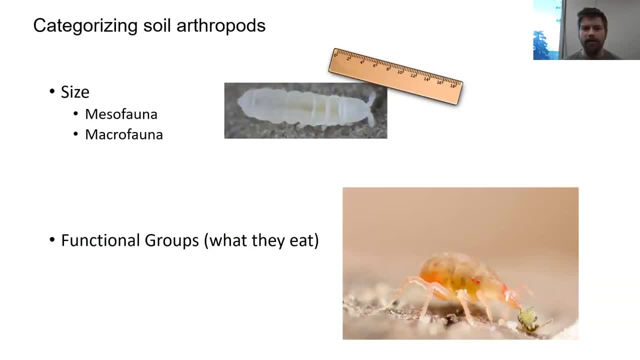 about how we talk about, how we categorize soil arthropods, And there's primarily two main ways. The first is by size: They fall into groups called the mesophana and the macrophana. And then the second way we talk about arthropods. 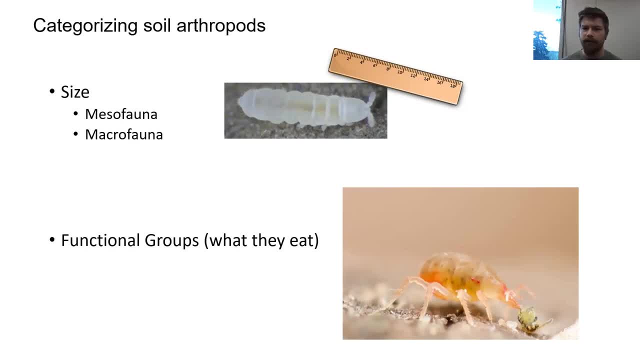 or think about. their categorization is by functional groups, which I alluded to earlier, And that just basically means what they eat. You can see here this example: This is a predatory mite here eating a springtail. So this would be an example. 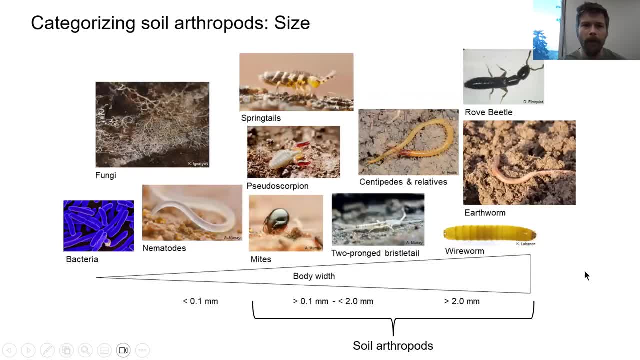 of what they eat. So this would be an example of a predator functional group. All right, so let's talk a little bit about size. As I mentioned, soil arthropods are categorized as the mesophana and macrophana, And we categorize them based off of their body width. 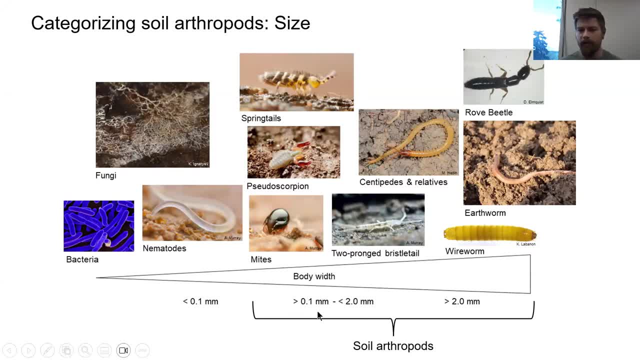 So mesophana are animals that have a body width greater than 0.1 millimeters but less than two millimeters. So again, these things are like springtails, mites, those two-pronged bristle tails. pseudoscorpions are another example of a mesophana soil arthropod. 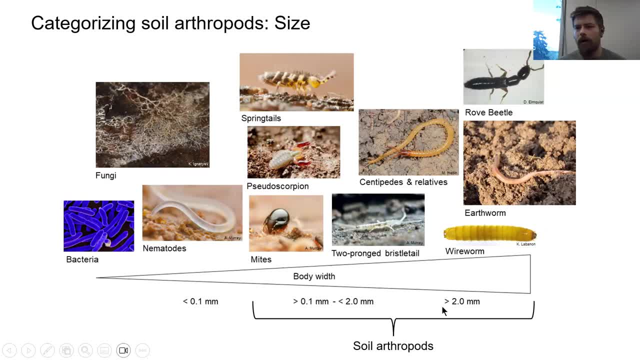 And then we get up into the macrophana as well, which include animals that have a body width greater than 2 millimeters. So things like beetles, wireworms and earthworms would also, although they're technically not arthropods. 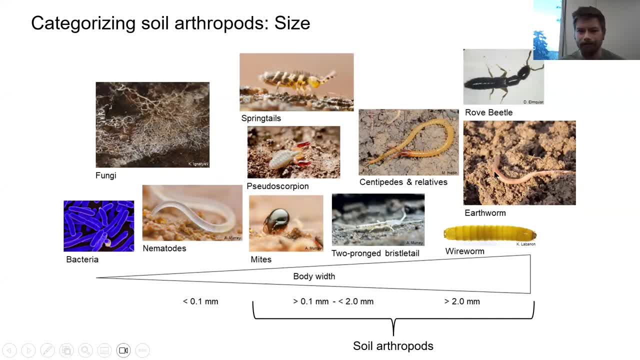 earthworms would also fall into the category of macrophana. And when we think about these less body width of less than 0.1 millimeters, these are things that are the micro fauna, things like soil, microbial communities, bacteria, fungi. 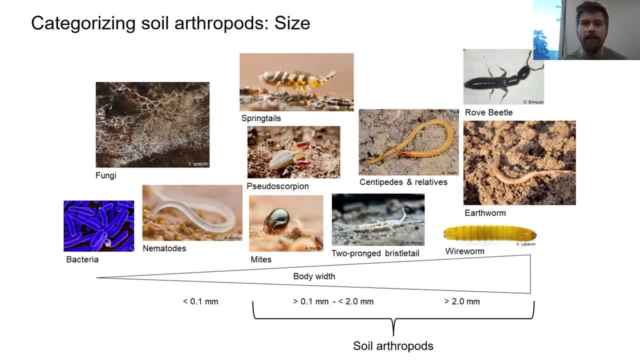 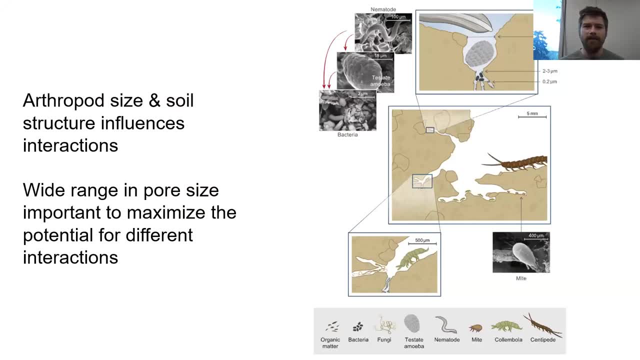 as well as nematodes, would fall into that size category. And thinking about size is relevant because the arthropod size, as well as the structure of the soil, is going to influence their interactions, right, So it's really the interactions between arthropods. 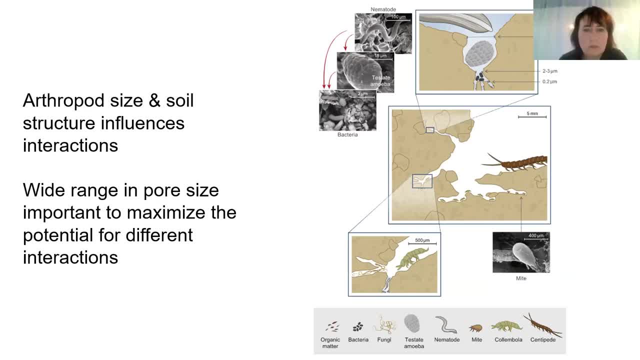 between arthropods with the soil right- pods and their food source, like fungi that are driving a lot of these ecosystem services like decomposition, nutrient cycling, and the soil structure is really important in influencing these interactions. and so when we're thinking about like management practices, practices that 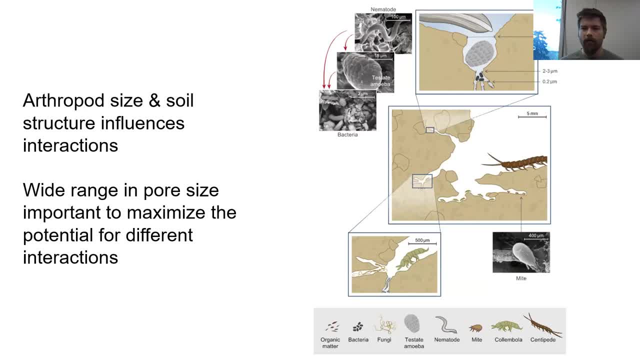 encourage a wide range and core size are really important to maximize the potential for these different interactions that are fueling ecosystem services that are are taking place in the soil. so you can imagine if you had a soil that was heavily compacted, really reducing the pore space. that is. 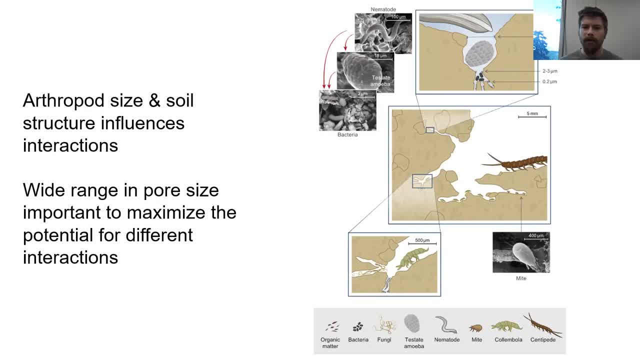 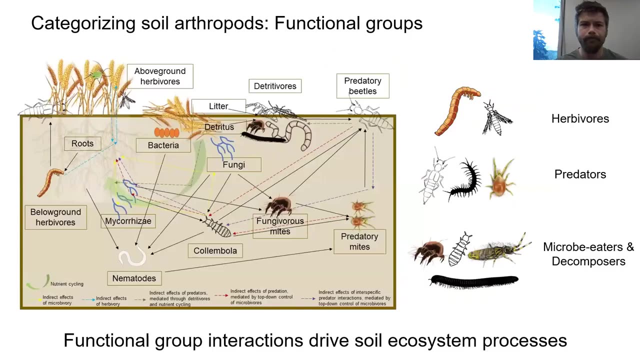 available for these interactions to occur, you might lose out on some of the ecosystem services that these soil arthropods are providing. so thinking about arthropod size as well as soil structure is, uh, is really, um, really important. all right, so now moving on to talking about categorizing soil arthropods as a function, 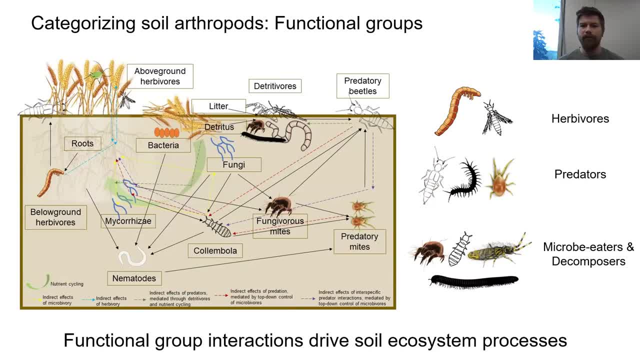 different functional groups. um. so, as i mentioned, these functional group interactions are really what's driving ecosystem processes in the soil. i've got this kind of complicated food web here to the left, but basically we're going to just talk about three main functional groups: the herbivores, predators, as well as the micro beaters and decomposers, and i'm going to go through here. 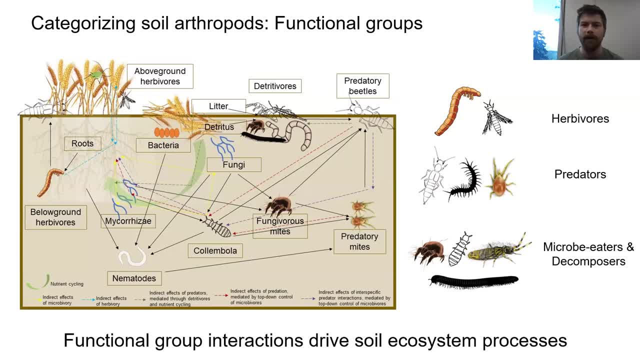 and share some pictures of some of the different functional groups that we're going to be talking about, as well as the micro beaters and decomposers, and i'm going to go through here and share some pictures and some fun facts and videos about members of each of these different groups, and 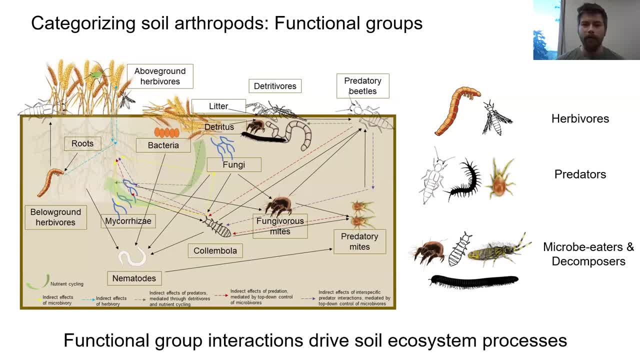 all of the critters that we're going to highlight here are actually from the soil arthropod communities collected from the agricultural systems here in the pacific northwest, so it's not like anything that's- uh, you know, found in the in the tropics or anything these things are. 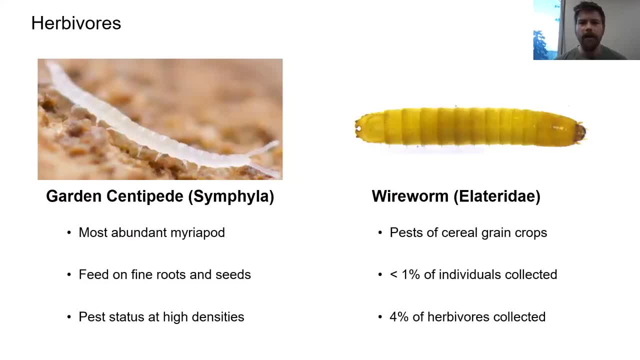 right outside our back door. so let's- uh, let's take a look at herbivores first. um, i'm just highlighting a couple, uh, herbivores here that were especially, um, either prevalent in our samples or economically important to producers here in the palouse. so the first one i'm going to highlight here are called garden centipedes, or 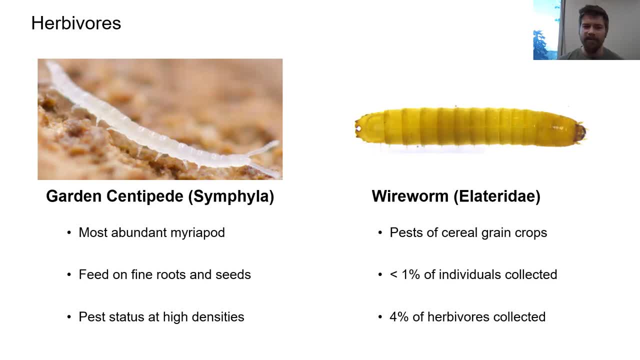 some filings. garden centipede is a little bit of a misnomer because these guys are not technically centipedes, although they're related to centipedes and millipedes. they're in that same group of myriapods and these some filings were the most abundant myriapod that we collected in our sample. 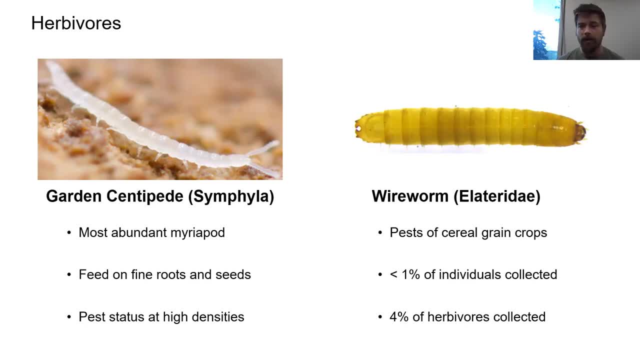 samples, um occasionally we would pull out a soil core and extract the communities from them and there would be, um you know, 50 or 60 of these guys in just a two liter soil sample. so they can be really prevalent. and they are herbivores. they do feed on fine roots and seeds and they can reach. 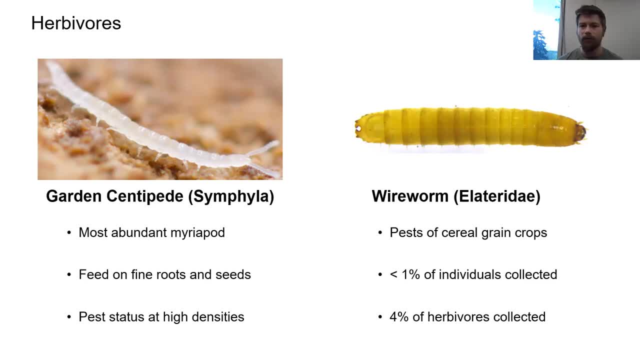 pest status at really high densities if they're not controlled by other predators in the soil. fortunately for us, throughout all of our sampling we really didn't ever find them at these high densities. that would prefer pest status to them. so they're. they're more of a- um, not really a. 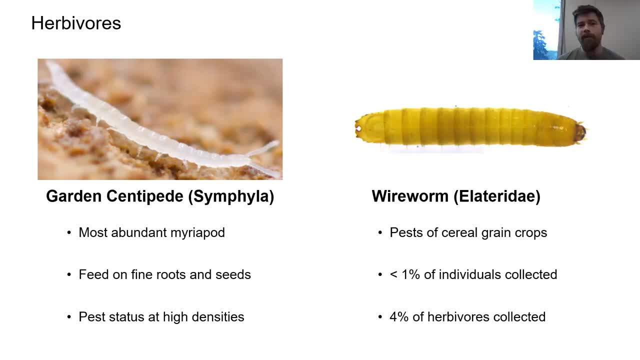 pest in in our ag systems? um, they are, they can be pests in like vegetable growing systems. so if you have like a small um scale like organic vegetable farm, um you know, these guys could uh, potentially be pests. but in our um cereal, you know, large cereal systems they they don't really reach. 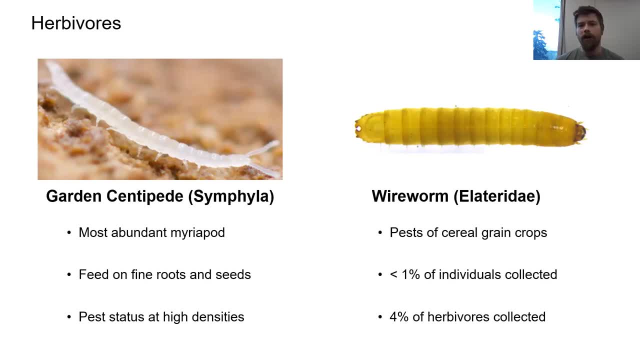 pest status at all. so, um, talk about pests. uh, moving over to the wire work, uh elatera day. so these guys are um pretty well known to a lot of producers here on the flus as their pests of cereal grain crops. um, one thing that might be uh positive news is, out of all of our sampling, those over 120 000 arthropods that 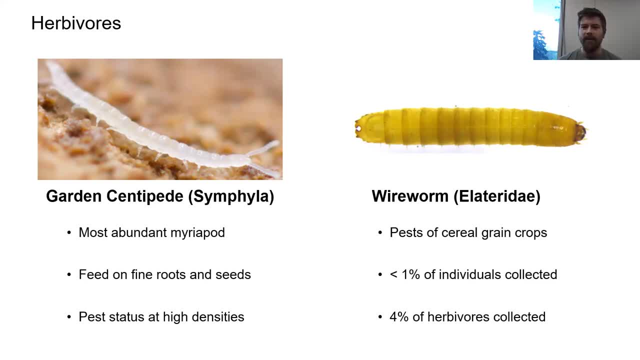 we've collected. wire worms represented less than one percent of all the individuals collected, and only four percent of the total herbivore functional groups collect that we, that we collected so um, while they they are pests um we we did not actually find them in in large numbers throughout all of our sampling in uh numerous cereal crops um over the past four. 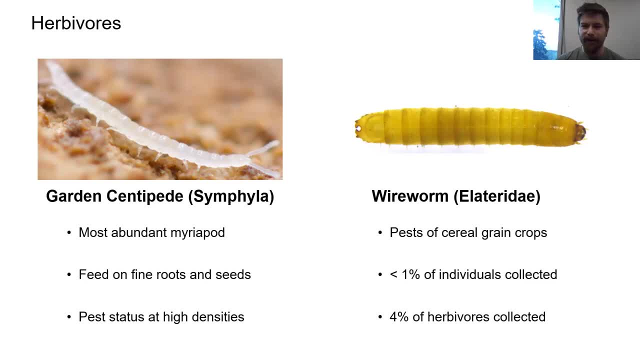 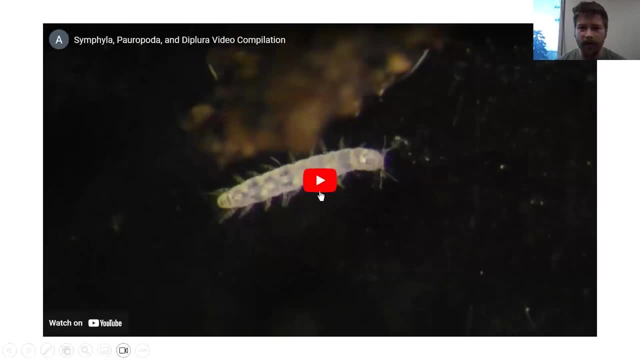 years. so you know, maybe that that might be considered a a good thing, depending on- uh, you know what you're growing and who you are, so i'm going to share a just a quick video here, um, just of some filing here in action. so this is an. 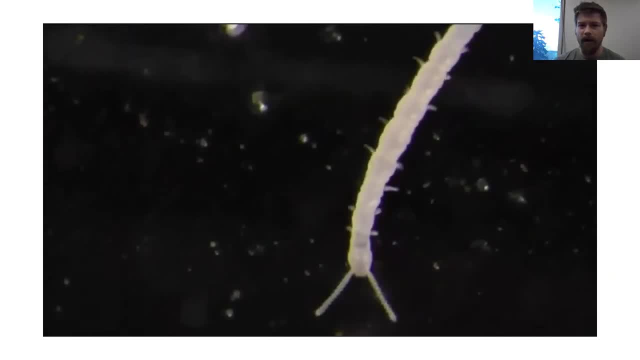 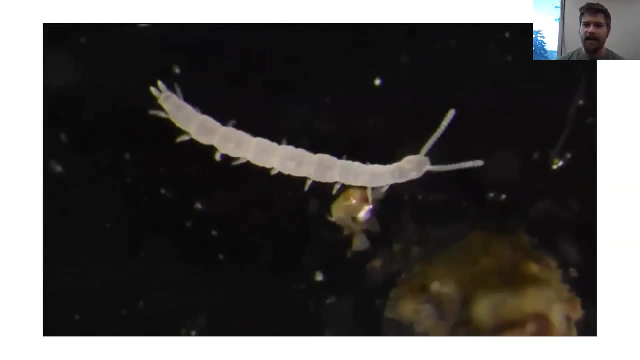 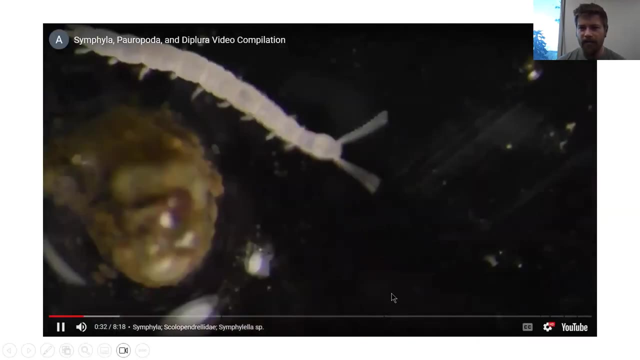 uh, a youtube video again of a garden centipede, um, and this is actually the, the same species that we have here, um, on the flus, so you can kind of see it's. it's got a similar morphology to centipedes and millipedes, um. you know, this is the head right here with the antennae. you can see that there are. 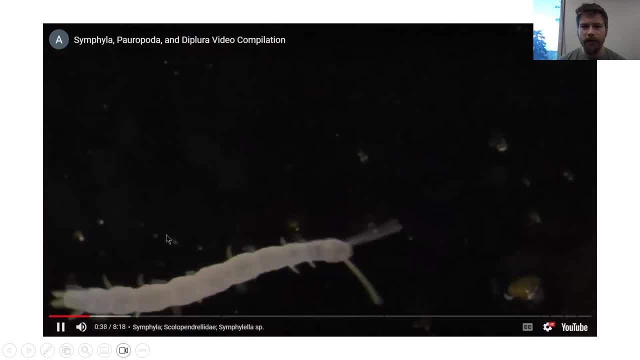 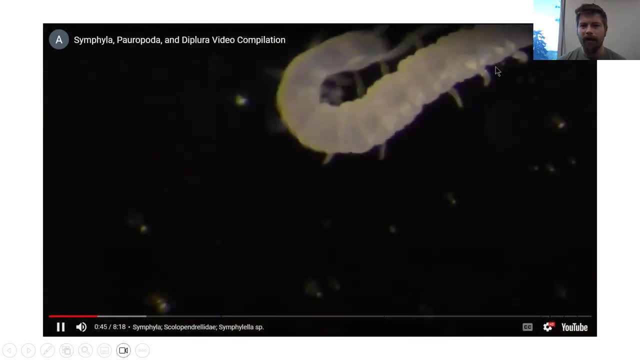 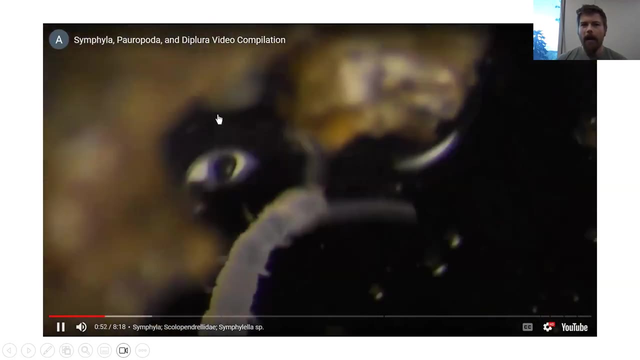 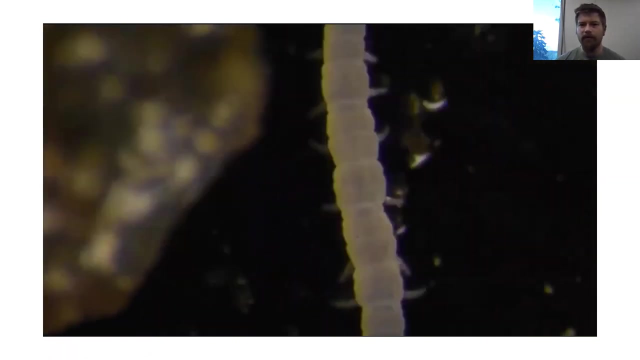 legs on each segment here, as well as two, um sorry, moving around a little bit- two of these uh protruding um appendages on its backside here, so you can get that back in focus. they're always white, they're always eyeless um, and this just is representative of their, their habitat, you know, living uh below the ground. 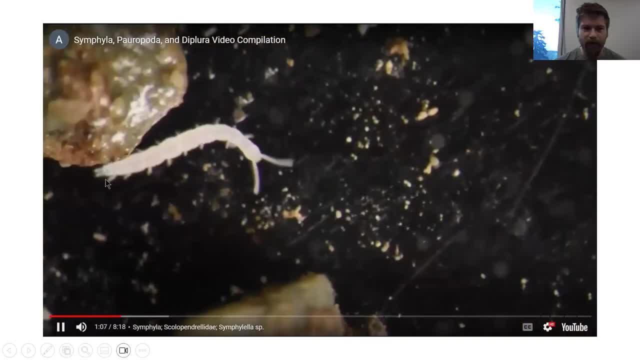 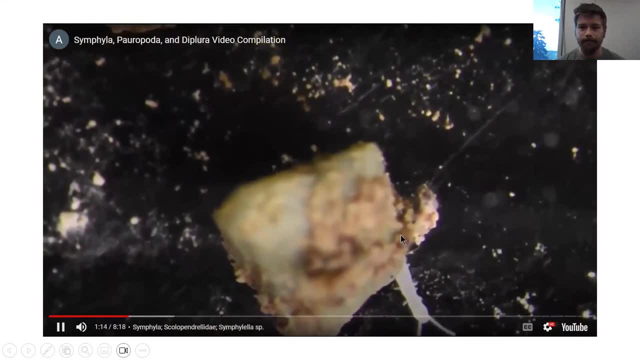 that's a nice video. there's those appendages that i was trying to point out there that was right on the back, kind of those two, two pointy, uh appendages off the posterior there. so that's uh, yeah, that's a symphylin again and that's the same species that we have. 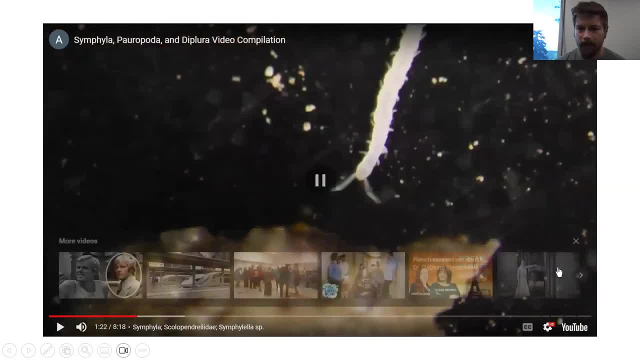 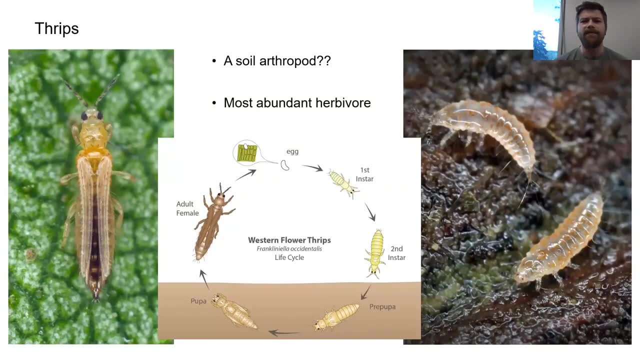 um, here, here in the inlands of the northwest. so i'll move on here to our, our next group. um yeah, thrips. so i wanted to talk about thrips for a second, because when i first started out- uh, this project, you know, knowing a little bit about thrips as foliar pests, 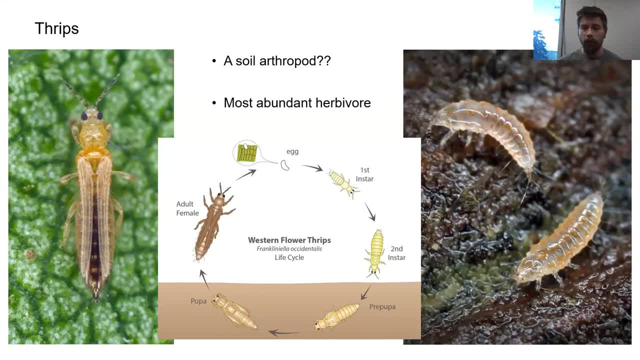 i really never expected them to find them in our soil arthropod samples. however, they were, in fact, the most abundant soil arthropod herbivore that we collected throughout all of our sampling and looking into this a little bit more, i've got the life cycle of thrips up here on the screen. 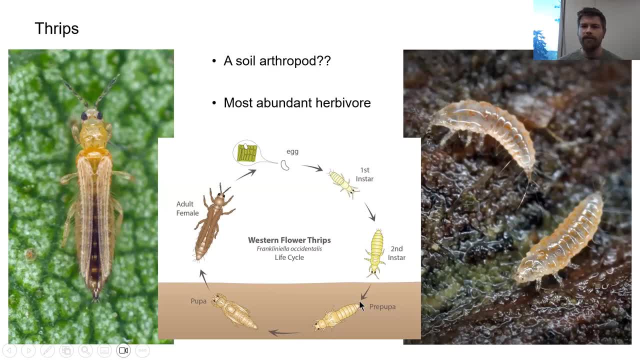 you can see that, right before they are going to turn into an adult, they actually will drop off the plant and spend this time basically turning into adults in the soil, and so this is actually, you know, one area where they can be targeted for potential biological control, because there's lots of predators in the soil, so the thrips when they drop into this, uh, the. 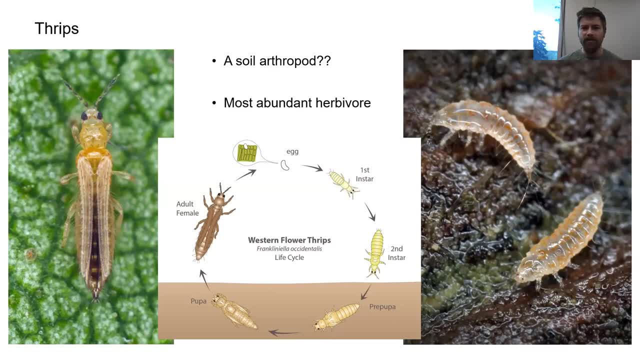 soil. during this portion of their life cycle they're at a really vulnerable stage. so, again, having a solid predator community in agricultural systems may help give the potential for biological control of thrips during this vulnerable stage of their life cycle. so a little bit of a surprise to me to see these guys in our soil samples, so much. but 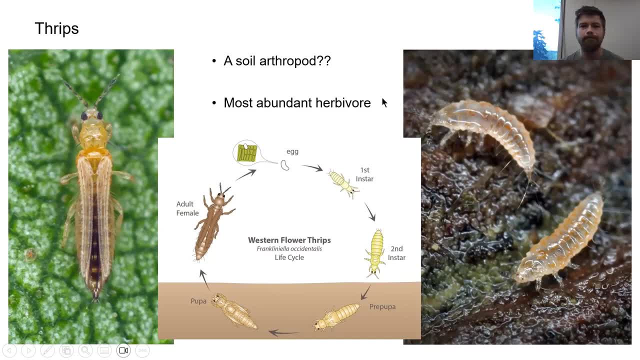 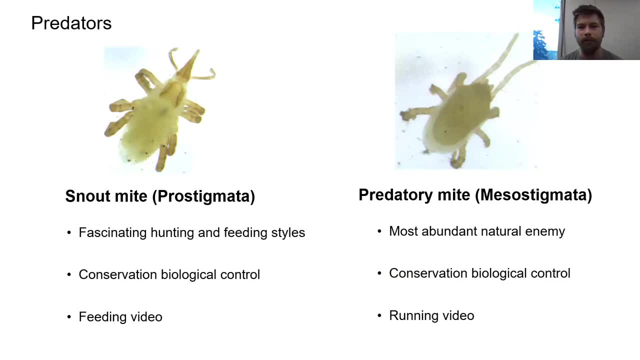 looking at the life cycle, it definitely makes sense that they would be there. all right, so moving on to uh, to predators, our next functional group: predators- these are some of my favorite guys. here we're looking at two predatory mites. the predatory mites are a really large portion of the soil- arthropods that we sample from agricultural systems, and i'll just 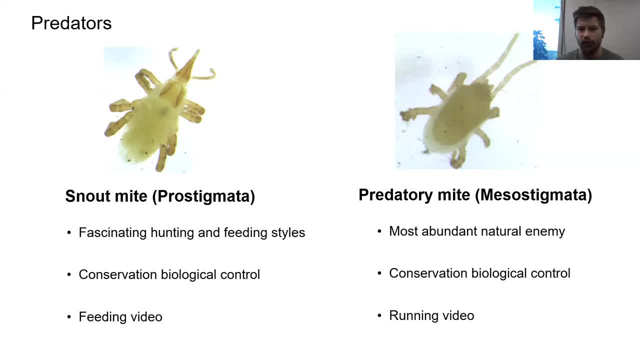 spend a little bit of time talking about that, but i want to talk about that a little bit more in the future. so we're going to be talking about a couple, um important uh groups here. so the first one we're going to talk about are the snout mites or the prostigmata. um, you can tell they're uh called. 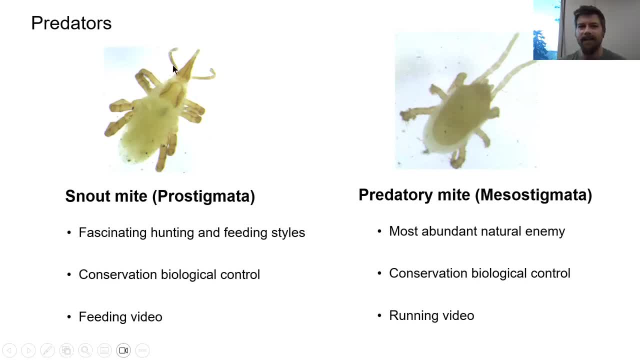 snout mites because of this uh, you know snout, that uh is formed here, um, on the the front of their head. these are actually the mouthparts that are colliserate. so they will actually rub these guys together, um, and that's how they will, uh, pierce the, the skin of, or the cuticle of, some of their prey. 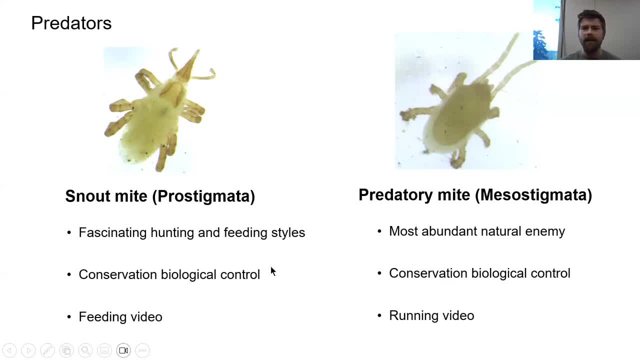 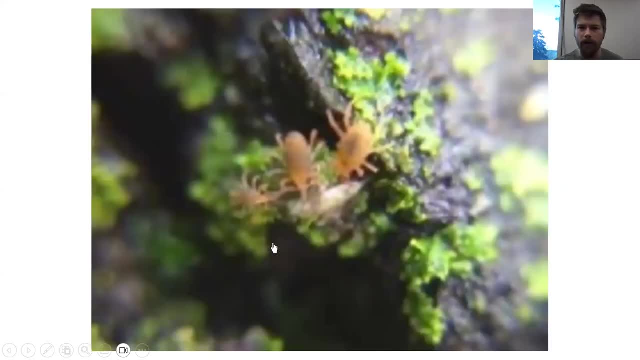 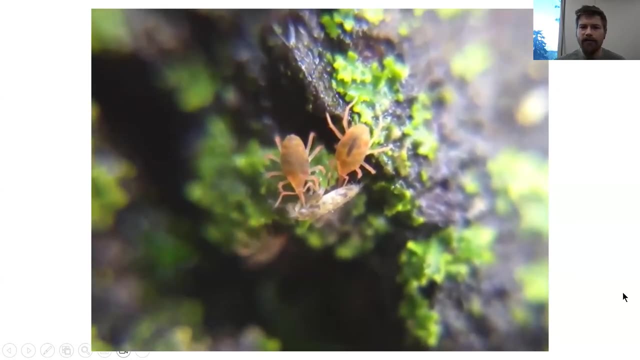 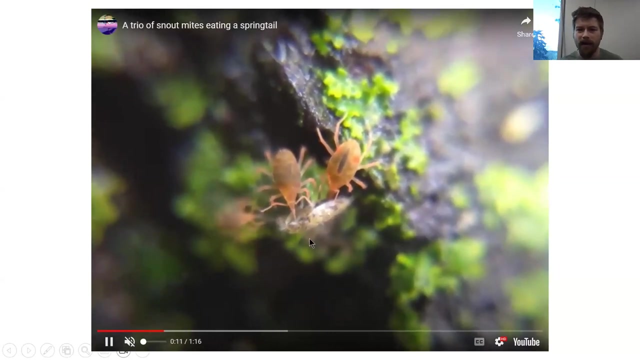 and so these guys have really fascinating hunting and feeding styles and again, they're an important part of uh conservation biological control program and i'm going to just show a quick video here of some predatory mites- snout mites consuming a columbola. so you can see here that snout is uh penetrating the integument of this. 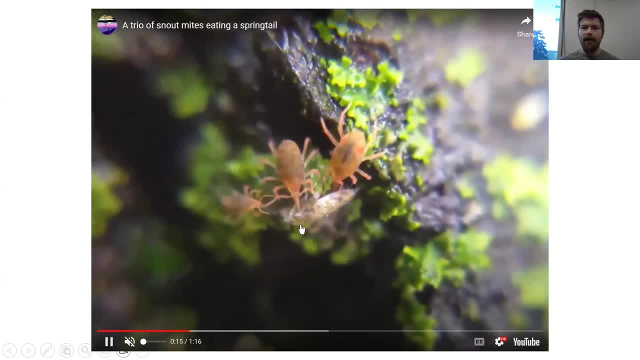 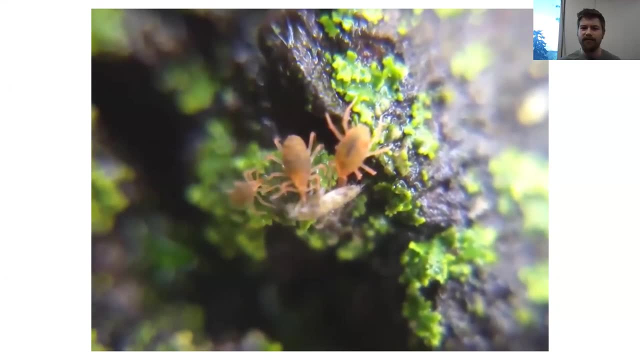 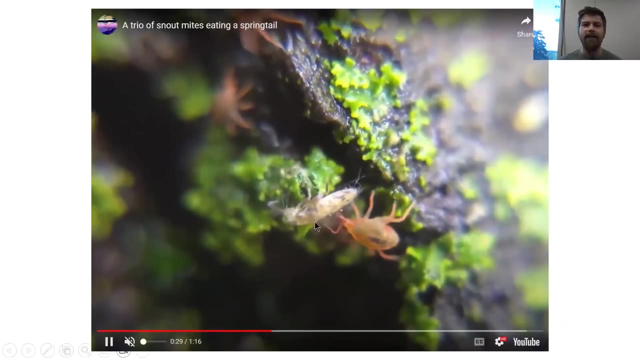 spring tail. um, and basically what they're doing now is they're injecting a kind of nasty cocktail of different enzymes and saliva into this spring tail and they're basically turning it into a smoothie on the inside. so they're smoothifying it and then they're- uh, they're sucking the the smoothie. 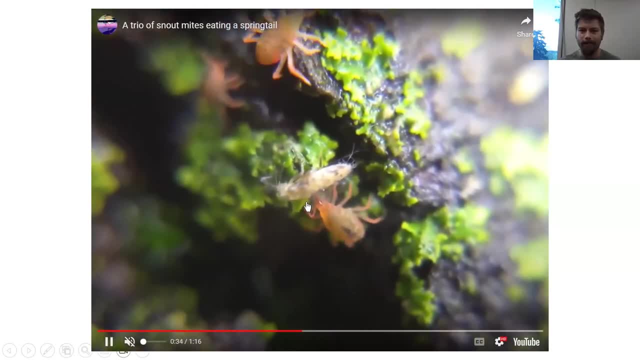 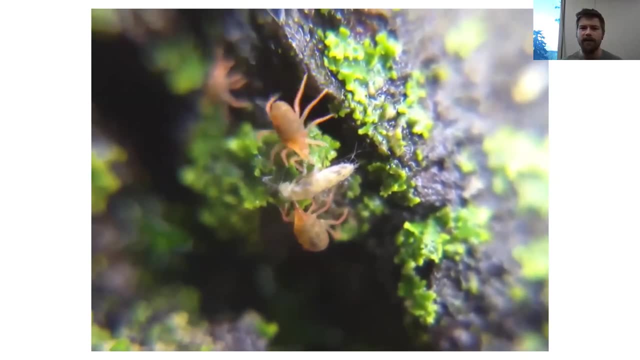 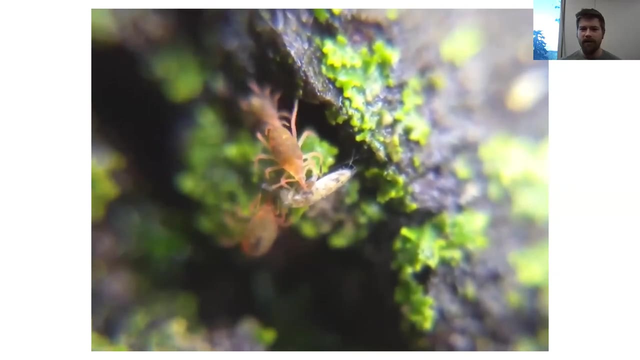 uh, of the what is now the columbola out, um, and so they're multiple, you know, mites feeding on this columbola, and i really like showing these videos because, um, you know, these are, these are the interactions that are occurring in the soil underneath our feet, even though we don't see them. 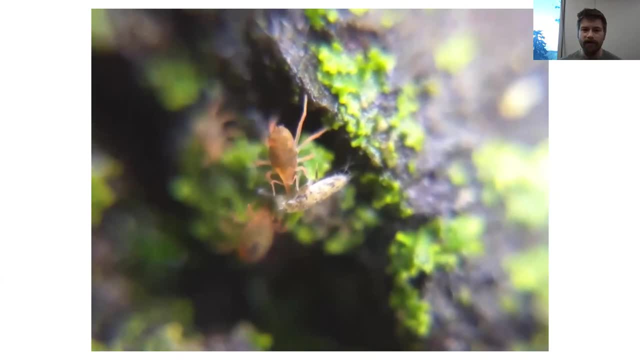 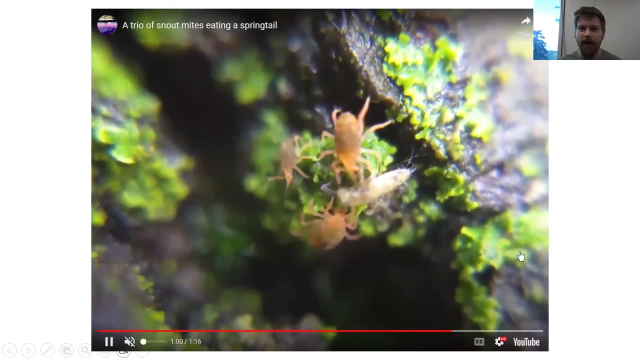 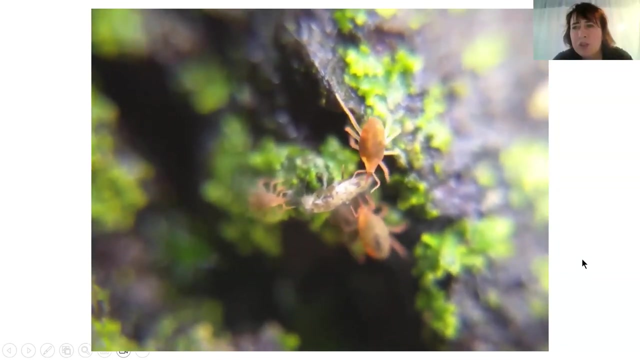 it's a really active place and- and this is this is some of uh, the stuff that's happening down there. so, yeah, some snout mites feeding and, you know, potentially competing with each other for this, uh, this spring tail resource. yeah, that's a very interesting video of that. yeah, these are uh. 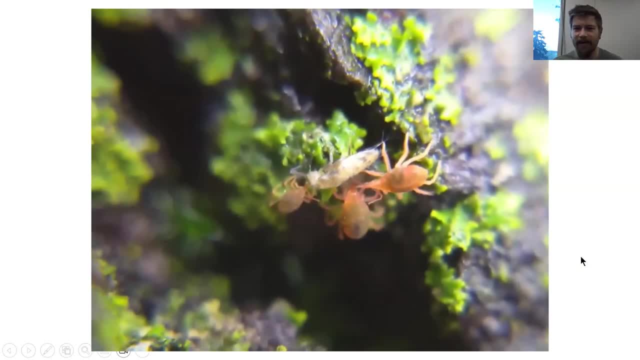 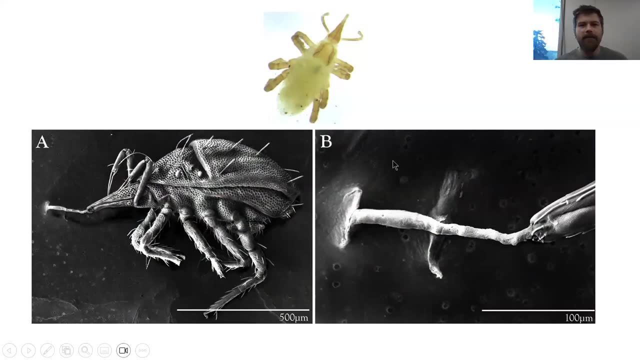 these are some of my favorite- uh favorite- mites that we uh that we get out in our uh ag systems all right, and i mentioned that they uh had some pretty fascinating hunting styles, so i wanted to highlight um another kind of fun fact about these guys. um, what we're looking at here is a scanning. 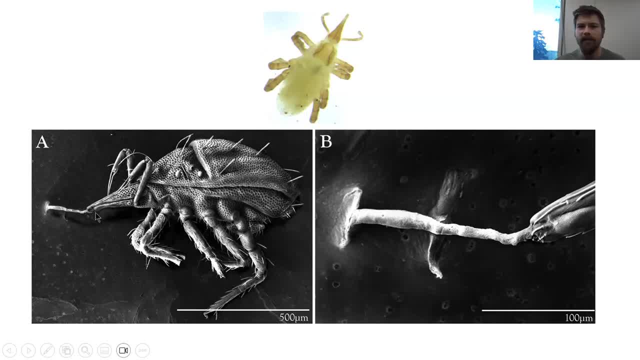 electron micrograph of what's called the silk capture mechanism. so mites are arachnids similar to spiders. they have the potential to produce silk, and these guys will actually produce silk out of their snouts that they can actually shoot um at a potential prey. 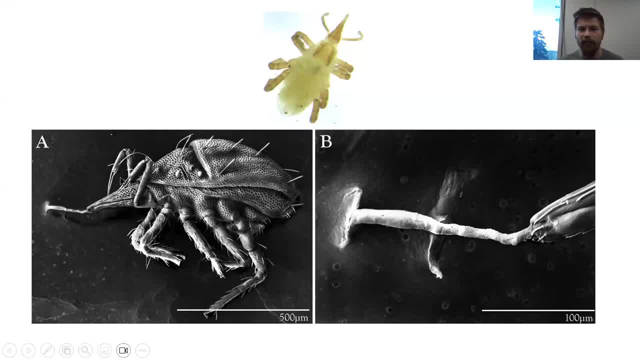 to capture it. and then they use these, uh, these raptorial pedipelps is what they're called. they're part of the mouth parts, raptorial pedipelps to you know. go and finish the job, turn it into a smoothie and, uh, and have a meal. so again, some fascinating hunting and feeding styles that occur down there. 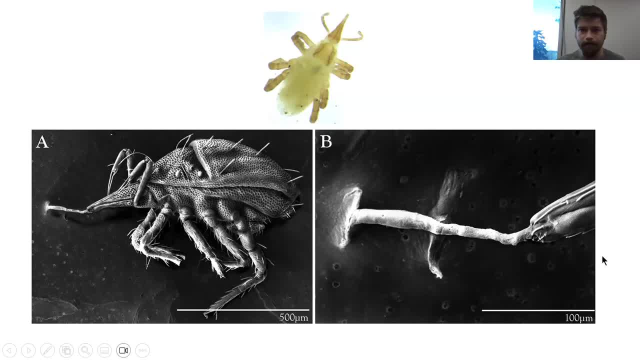 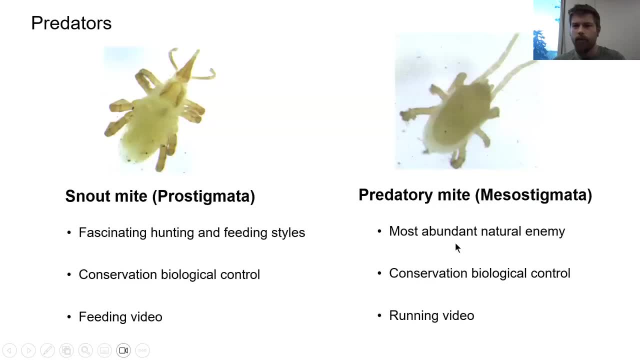 in the soil, where we might never think that these things are occurring. all right, and uh, this next video. i'm actually going to jump back here really quick, so next i want to talk about these other mites that are called, uh, the mesostigmata. i kind of think of these guys as the wolves of the soil. 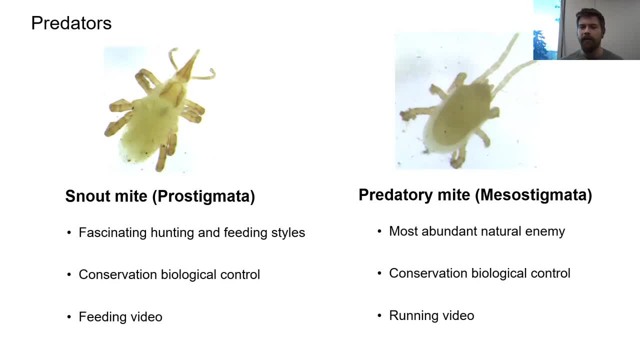 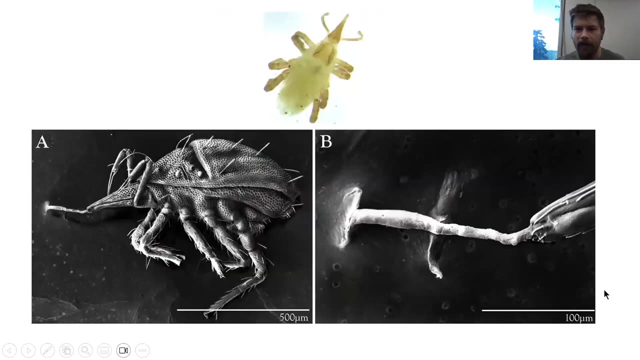 um, these were the most abundant natural enemy or predator that we recovered from our soil arthropod sampling and, again, they're important part of conservation biological control programs and these guys are readily identified by these forward-facing legs which they use to capture prey, and i'm going to just share a quick video of them, um, running around. basically. so this is the. 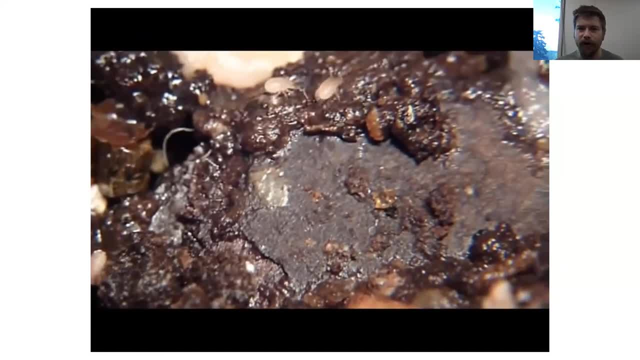 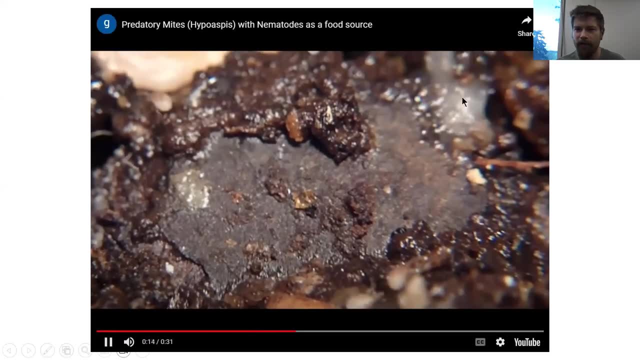 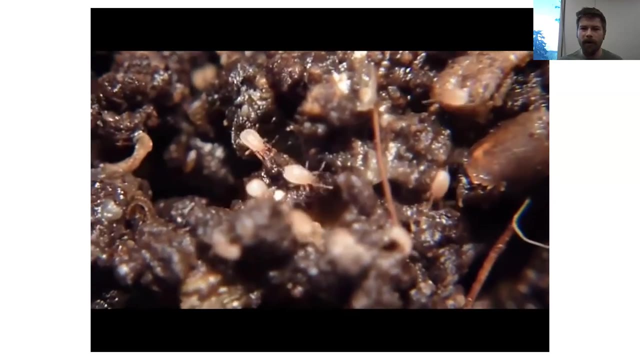 a video of these predatory mesostigmated mites. you can see those front legs, uh pointed out in front of their body there, um, and what we're looking at here actually this uh kind of moving goop is, uh is a pile of nematodes, um. so these guys are predatory mites. they eat arthropods, but they 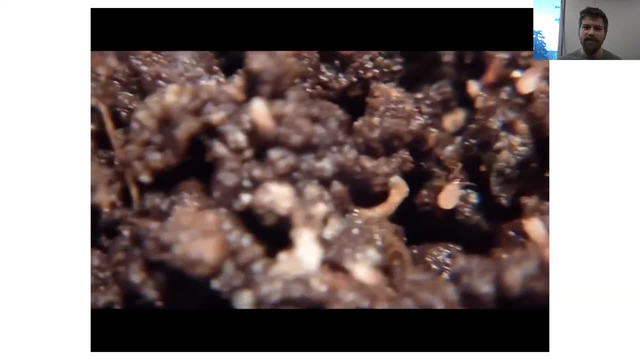 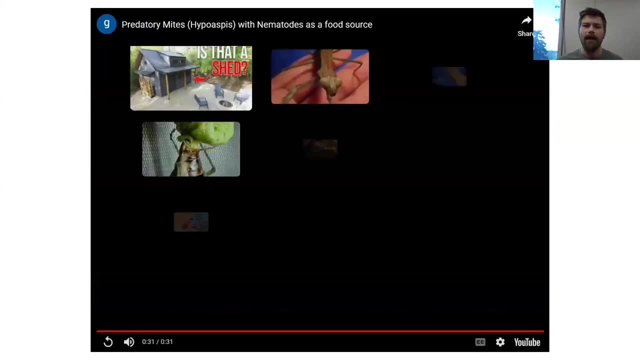 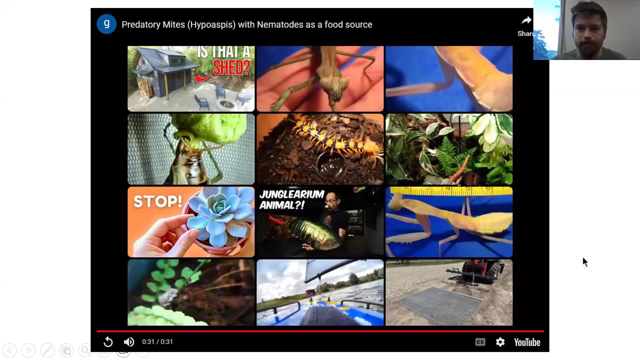 also eat nematodes and they can consume um thousands and thousands of nematodes. so they can be important in terms of uh, you know, helping promote suppressive soils and potentially um eating pathogenic nematodes that we don't want in our systems. so again, they're like the wolves of. 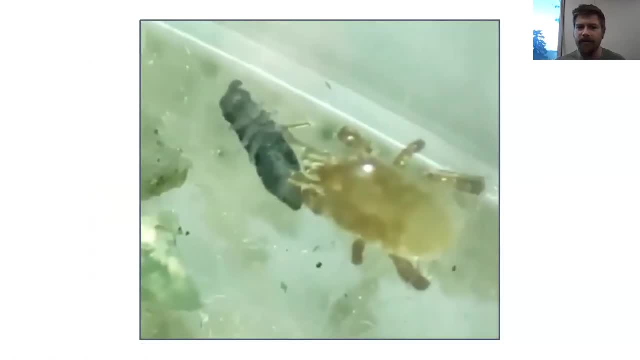 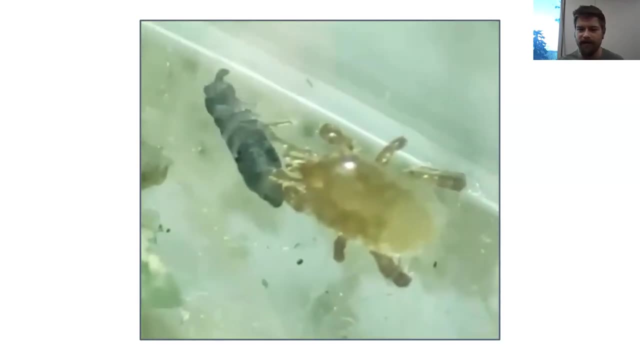 the soil. i i consider them. they're fast, they're voracious, and here's another video of a mite that's captured, a springtail, um, and it's uh, yeah, that springtail is about to meet its last moments here and that might's going to have a meal. 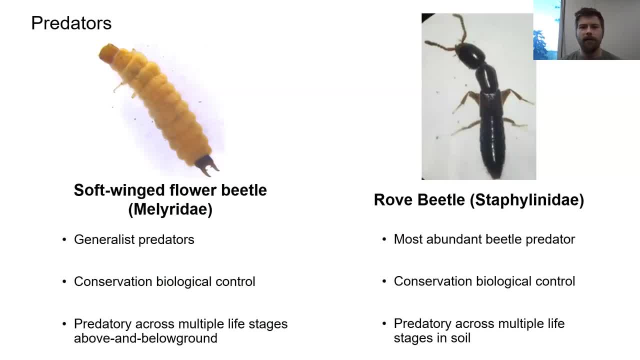 all right. so, moving on to some other predators, um, i'd like to highlight some of these, uh, these beetle predators that we're going to be talking about in the next few minutes, and then we're going to move on to some other predators. um, i'd like to highlight some of these, uh, these beetle predators. 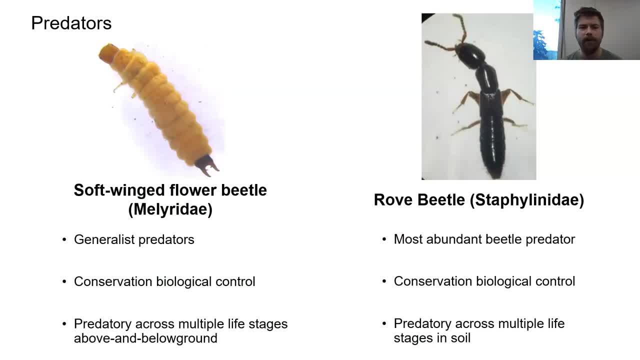 that we're relatively common in our soil arthropod communities. the first one i want to talk about here is the softling flower beetle, or malaria day. this is a picture of the larvae. these larvae live in the soil. they're generalist predators, which means they're not really picky about what they. 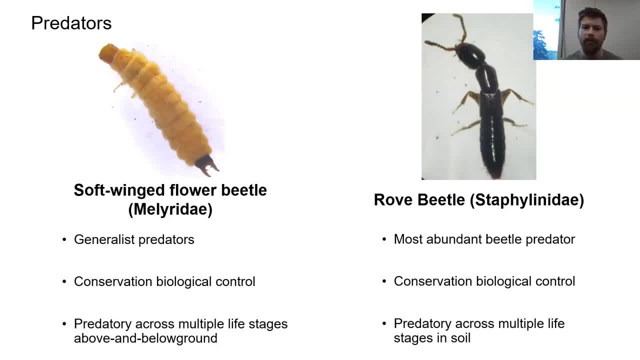 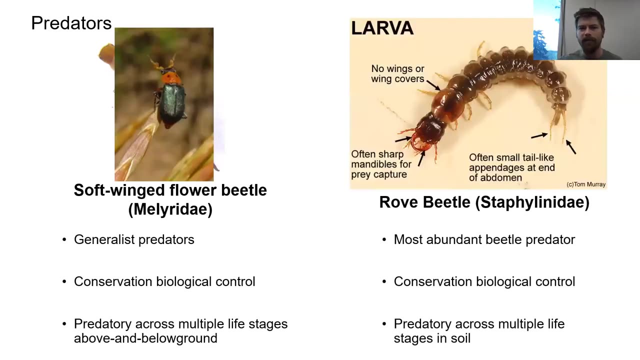 eat. so they're eating all sorts of things- again, very important part of a conservation potential conservation biological control program. and what's neat about these guys is they're predatory across multiple life stages, both above and below ground. so below ground they're predators as larvae, and above ground they're predators as the. 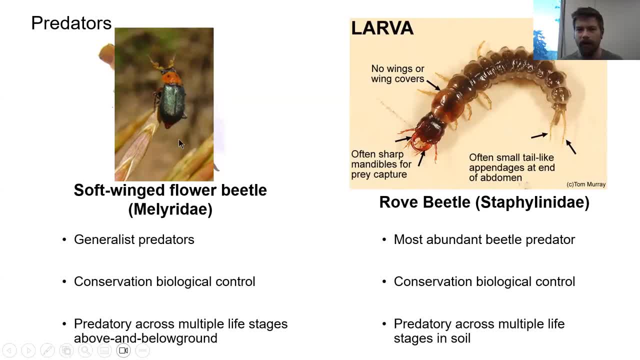 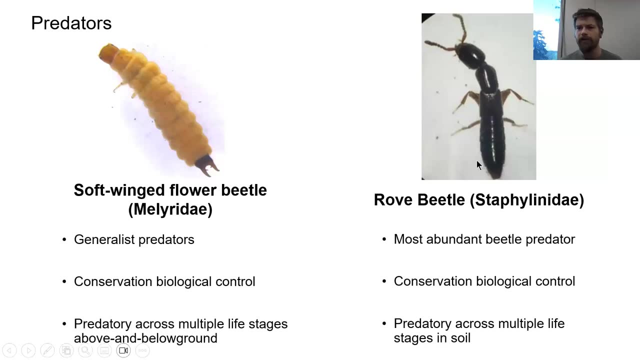 um, these colops beetles, which some of you may be familiar with, um, these guys are predators, uh, as adults, as well as larvae and um, so, yeah, you're kind of getting the best of both worlds, this potential for biological control in the soil as well as on your wheat plants. so, rove beetles, or 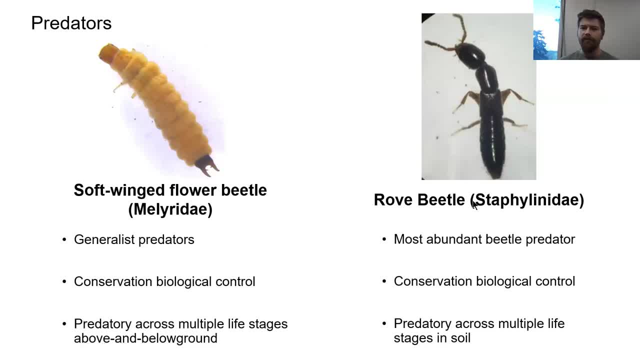 staphylinids. they were another uh, a very abundant beetle predator, again important for conservation, biological control potential, and they're also predatory across multiple life stages. but they primarily remain in the soil, so they're predatory as larvae as well as adults. this is a picture of an 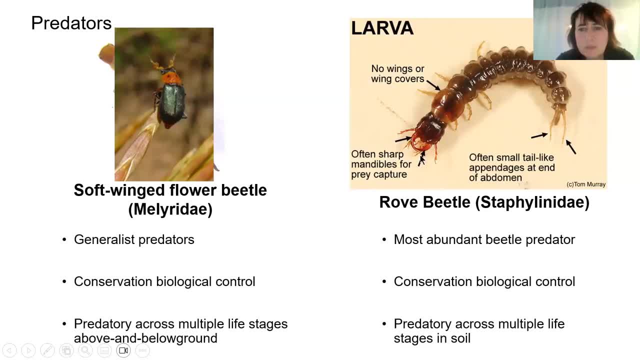 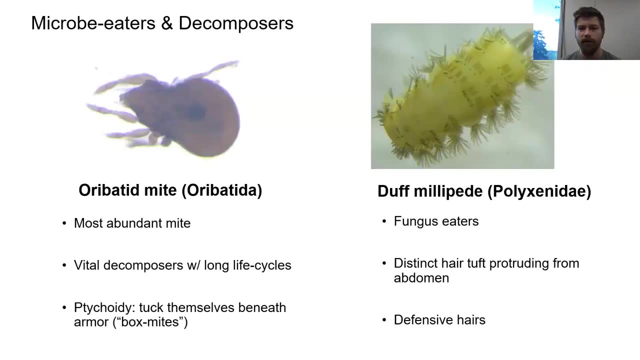 adult. and then here's a picture of a larva, and you can really see the predatory nature of these guys by looking at their really sharp mandibles that they use for for prey capture all right now, moving on to talking about, uh, another functional group, um, these guys are the most abundant functional group that we recover from our 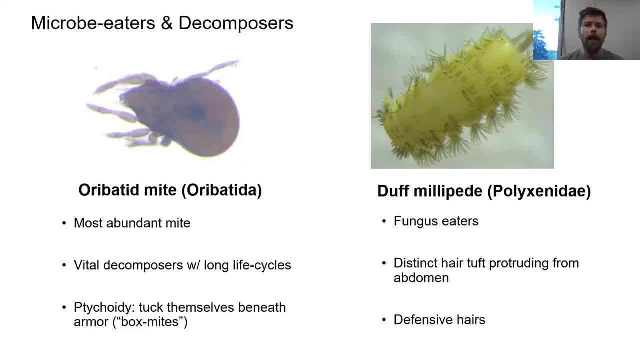 soil arthropod communities, um, and i'm just going to highlight a few critters here because they're they're kind of cool, um, and some of them, like this duff millipede, may not be, uh, familiar to to many folks. um, so the first group we're going to talk about are the orabatted mites. 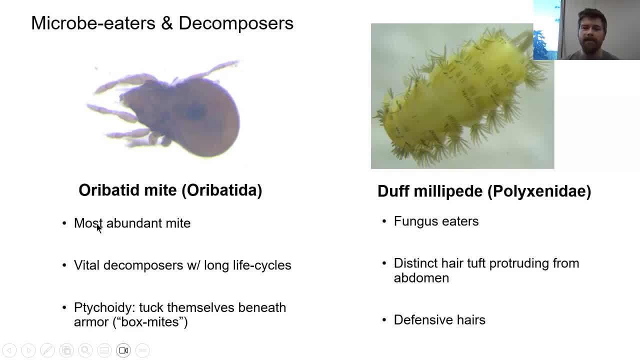 or the box mites um. these were the most abundant mites that we recovered from our soil arthropod communities. we would sometimes pull out our soil cores, extract them, and there would be hundreds and hundreds of these mites. i think the um, the number one most abundant species in a single sample were these orabatted mites and it was. 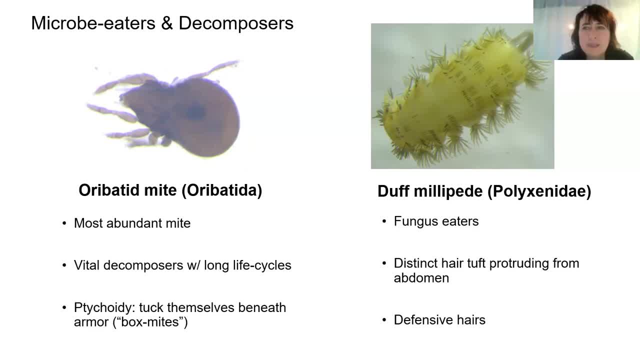 over a thousand individuals in one two thousand uh two liter soil core, so they can get into really really high numbers in the soil um and they're very important functionally. they're really important decomposers, nutrient cyclers may have really long life cycles um, and i like to highlight 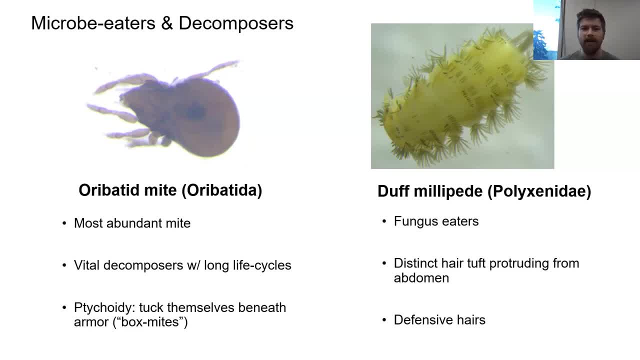 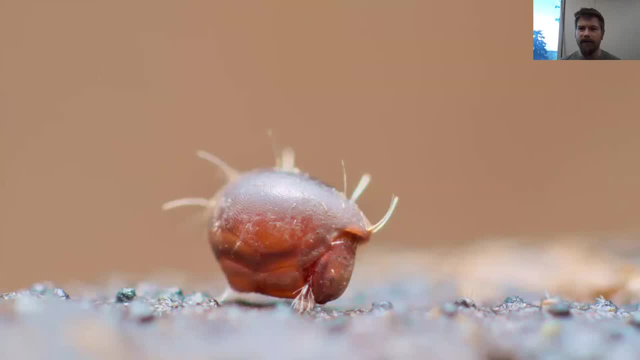 you know this fun fact: they're called box mites because they exhibit this behavior called hycoidee, in which they tuck themselves beneath their armor and basically look like this. so you can, uh, you can kind of see this mite has basically taken its legs, taken its head, fold it up into this armored ball here. so this is. 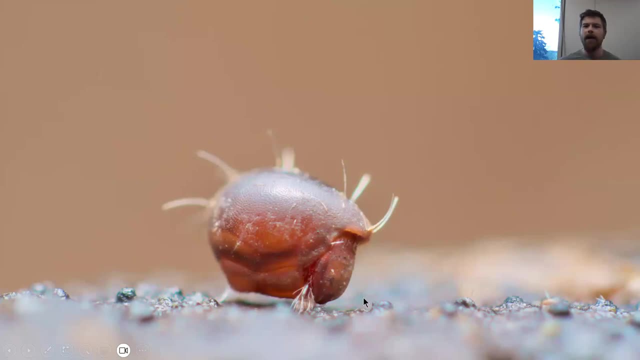 the head. um, just for some reference, um, and yeah, if you're a predator, uh or something trying to go after this, might you know this is a pretty good defense mechanism, especially if you're in the soil. you know where you can't readily return to the soil. you know you can't readily return to the soil. 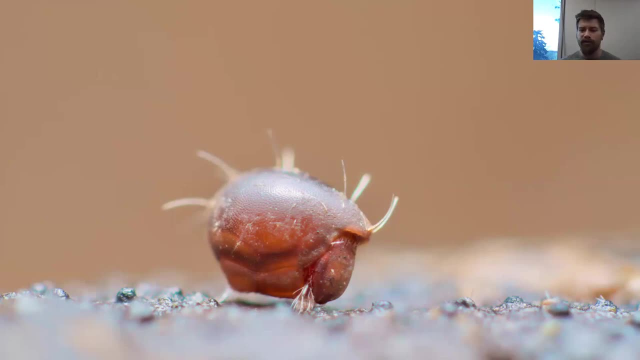 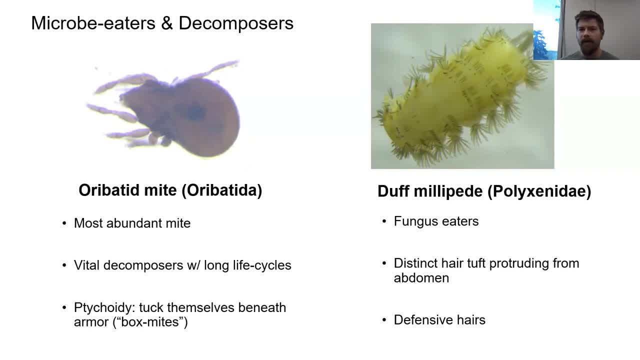 so duff millipedes are another uh decomposer that we find out in the uh soil arthropod communities and the ag systems here in the palouse. um, they're not very common, nowhere near as common as or a bad advice, but i like to highlight them just because they're kind of an. 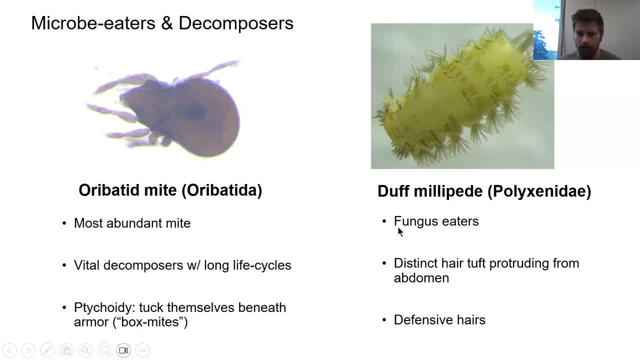 interesting critter. so these guys are fungus eaters um feeding on fungi in the soil, breaking up and liberating uh fungicide in the soil. breaking up and liberating uh fungicide in the soil and the nutrients that those microbial communities kind of take away um and liberating those. 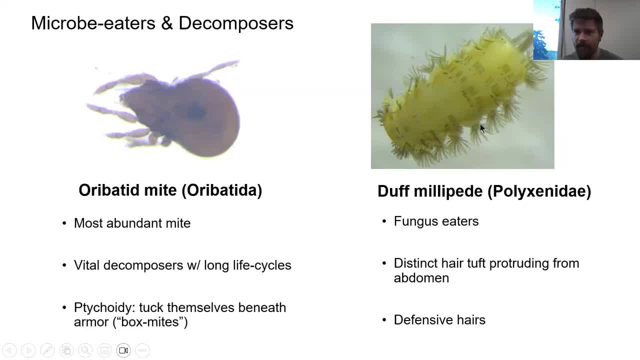 nutrients so that they are then available for plants. these guys are recognized by these distinct hair tufts that you can see here protruding from the abdomen, so they are millipedes. however, they really don't look anything like our- our traditional millipede right, and these hairs that we see here are are defensive. so, again, if, um, something is, uh, potentially going, 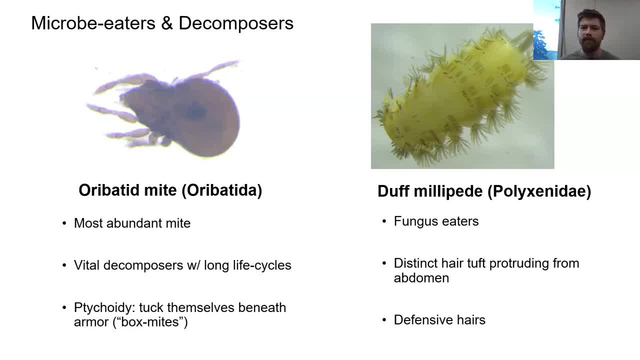 to eat or prey upon these duff millipedes. they have the ability to um have these irritating hairs that essentially will cause a predator to either give up or occasionally, as you can see, these hairs back here on the posterior end can be like eaten or taken and removed from the millipede and then 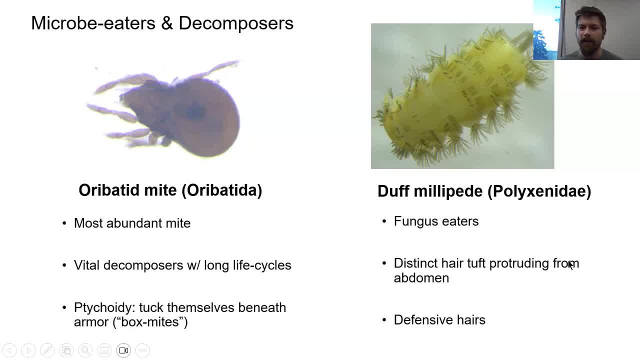 they can, you know, scurry away to safety, um. so it's kind of a a stakeout, so to speak, for for a predator to be able to attack them. so it's kind of an interesting critter that we find out in the in the soil, but they're not too common. all right, so moving on to another very important group again. 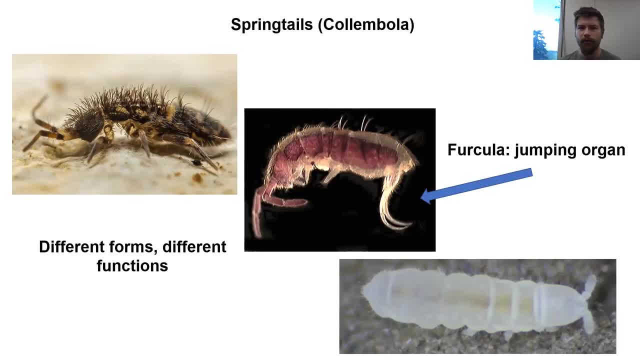 these guys are still in the microbeader decomposer functional group. these are the springtails or the columbula. again, these were outside of the mites. these were the second most abundant arthropods that we recover from soil, our soil arthropod community sampling. 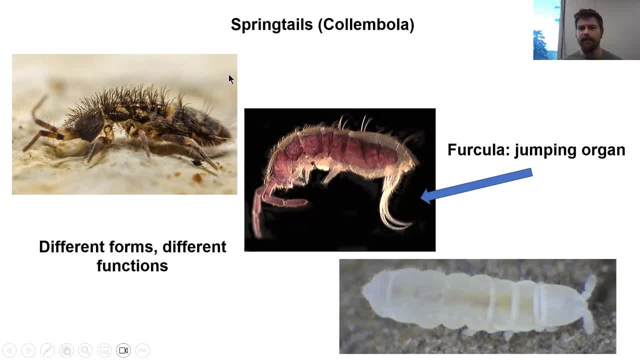 and they have many different forms, which kind of corresponds to their different functions, where we actually find them in the soil profile. and i'll just quick point out that they're called springtails because they have this unique uh appendage called the furcula, and we'll take a 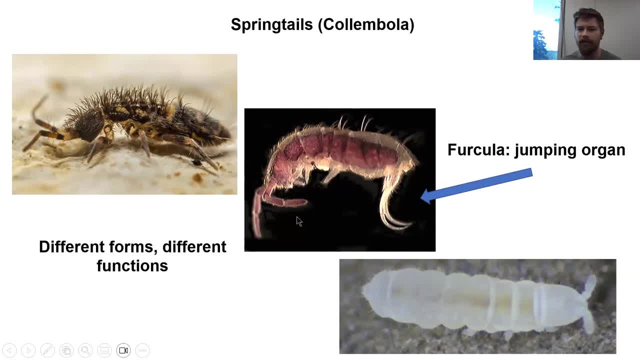 this is the jumping organ and we'll take a look at a video here that shows this in action in just one second. but i want to just quick go back to the different forms and different functions idea here. so you can kind of tell: i've got these three different springtail pictures on the uh. 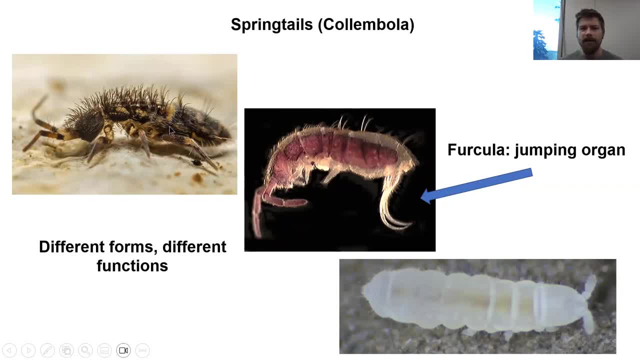 on the screen here and you might guess that you know this. this springtail here, this white eyeless, you know no pigmentation. this is a springtail that lives deep in the soil profile, whereas this uh springtail up here that has eyes, has some hairs, it's pigmented, has a very developed curricula. these guys are 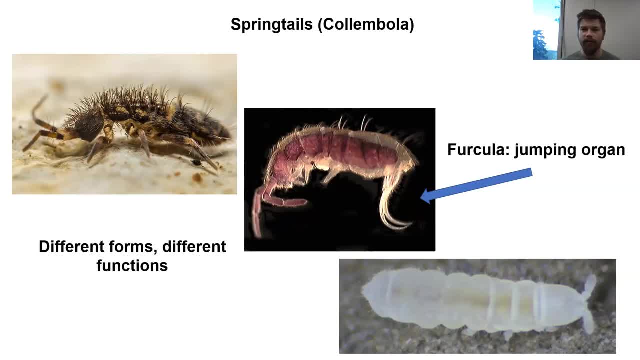 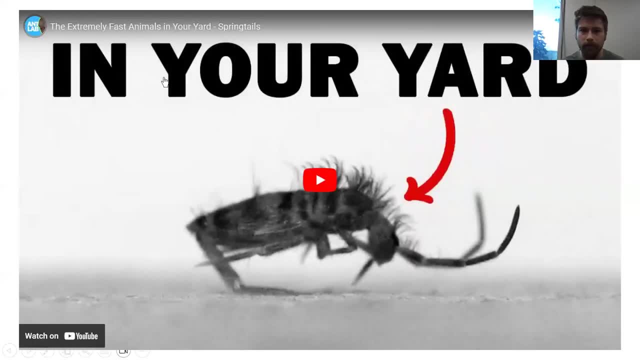 actually living on top of the soil, so these springtails are really abundant and they live in different areas within the soil, which kind of corresponds to to what they're actually doing in the system. all right, so here's a pretty neat video um of springtails in action. 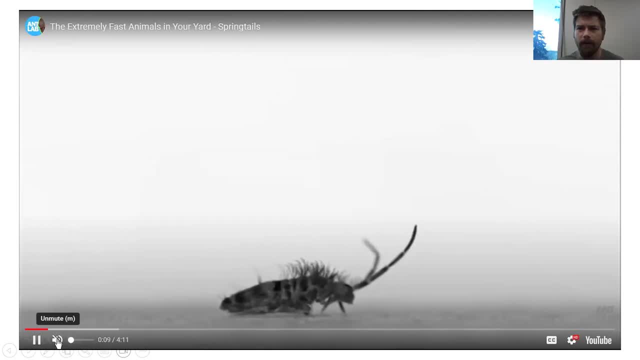 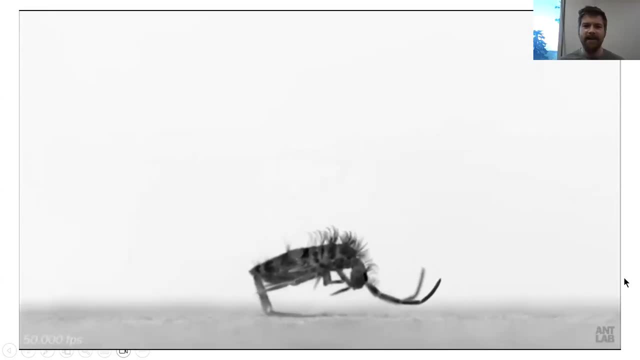 can you hear that uh narration in the video? okay, no, i think no problem. so, basically, what the what this guy is saying is that this is a a spring tail um springing at 50 000 frames per second. so this is really, really slowed down um. 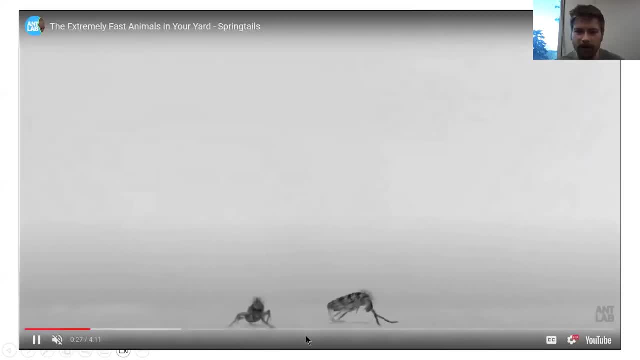 And I'll just kind of narrate along here when we get back to it So you can see. this is the furcula right here And basically what happens is when the springtail is threatened or needs to get away from a potential predator. 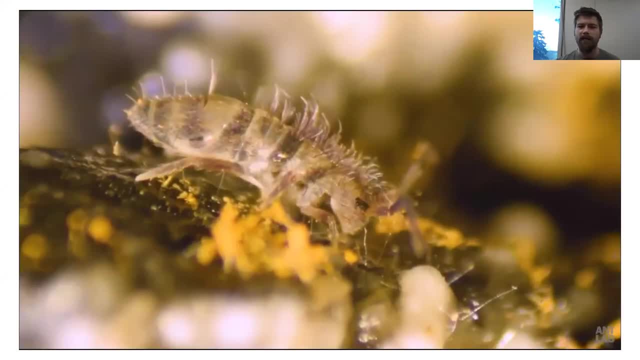 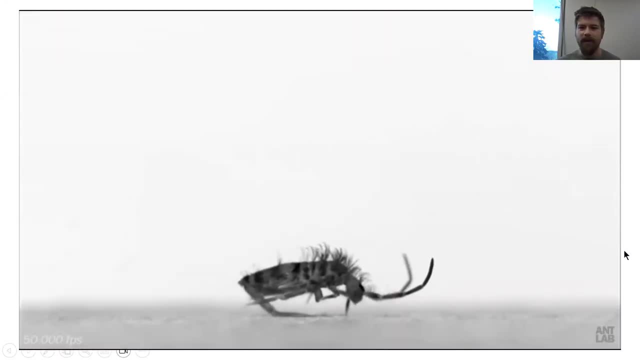 it will actually unhook this furcula which it keeps basically attached to the abdomen, And this furcula will hit the ground with some extreme speed which sends the springtail flying. So it's a really good way to get away from potential predators. 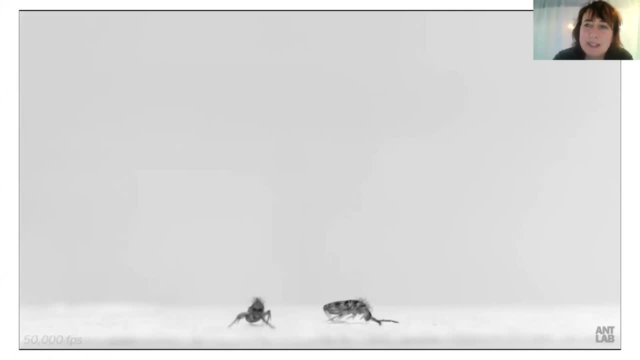 That's a nice slow motion version of that. Yeah, yeah, This is a really great YouTube video or YouTube channel It's called Ant Lab. for people that are interested, They have a lot of slow-mo videos of fascinating different insect behaviors. 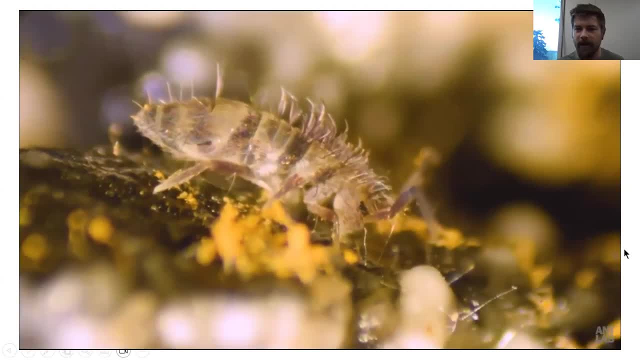 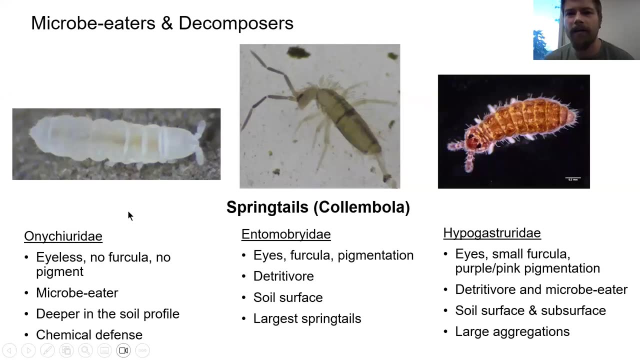 So highly encourage you to check that out. But yeah, they got some really nice pictures of the springtails, Okay. So I just want to again kind of go back here and highlight a couple of these critters. So first, looking at this springtail group, they're called onychurids. 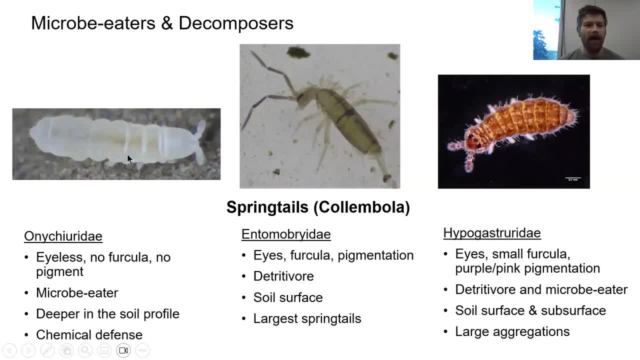 These guys are white eyeless. They don't have this furcula that we just saw. They don't need it because they actually live so deep in the soil and in these tiny little soil crevices and soil pores that they really have no use for a furcula. 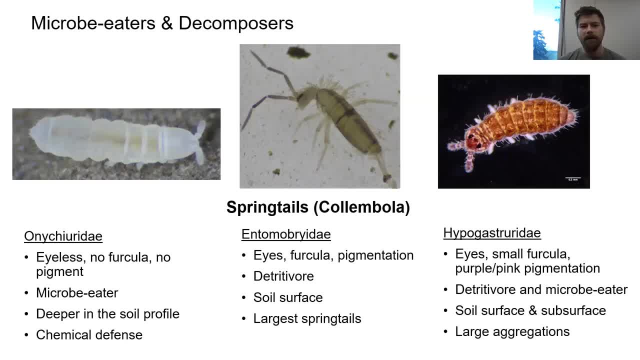 So they've actually lost it adaptively And these guys are microbial. They don't have this furcula to get away from predators. They primarily feed on fungi. They can feed on AMF And again, they live deeper in the soil profile. 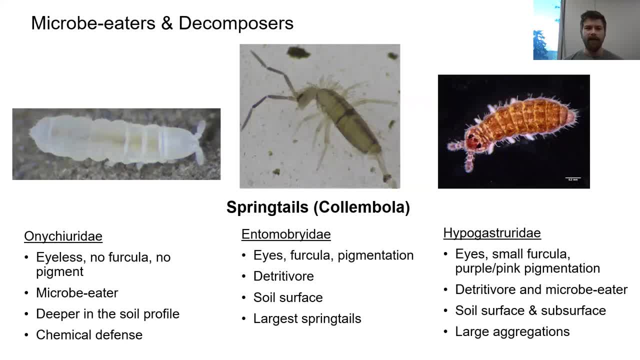 And because they don't have this furcula to get away from predators, they've evolved a different kind of defense, a chemical defense actually, And so they will actually exude a toxin when they're disturbed or something's coming up behind them, perhaps in the soil pore. 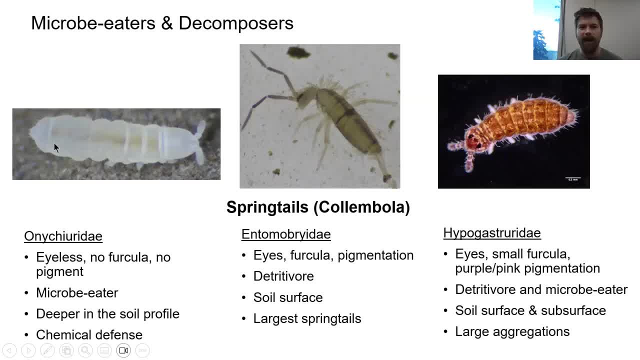 They'll actually exude a toxin from glands on their backs here, And so they will deter predators. So it's this chemical defense instead of a physical defense, so to speak, And so the next group I want to talk about here are the entomobreeds, or the elongate springtails. 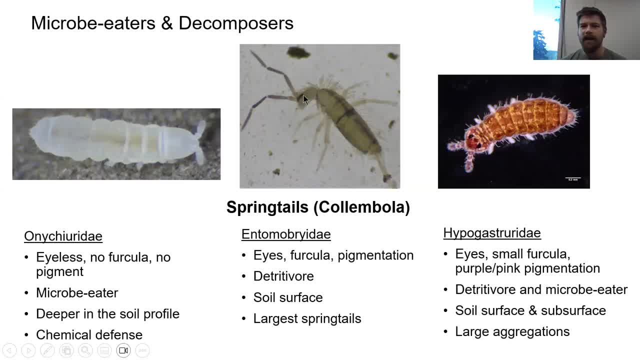 These are the guys that we just saw in that video. These have eyes, as you can see right here, This long developed furcula And they're pigmented and they have some nice hairs on their body. These guys are detritivores. 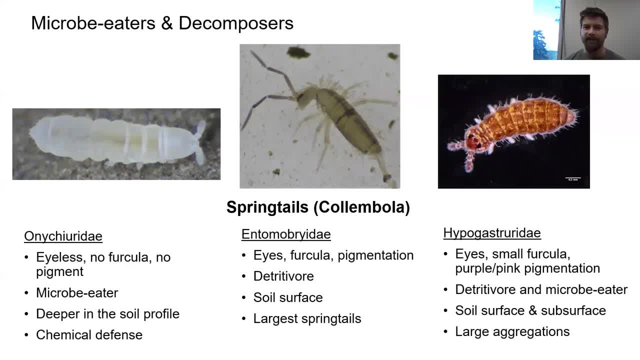 They live on the soil surface. They're primarily eating leaf litter Bacteria that are growing on the litter, breaking down, comminuting the litter and increasing the surface area of litter. that enhances the ability for microbial communities to colonize and then break it down further. 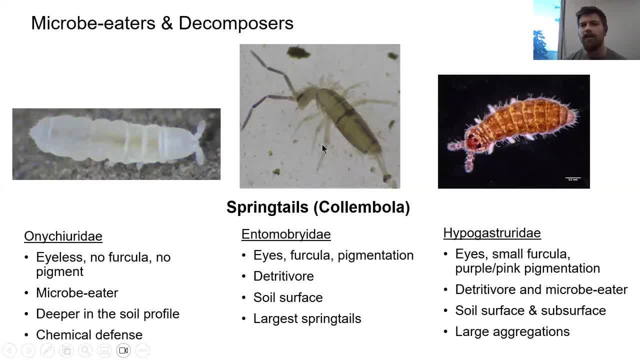 And so these guys are the largest springtails that we get around here. You know they're still pretty small, but you can actually see them with the naked eye. You can fit, maybe you know, 10 on your thumbnail- They're that big. 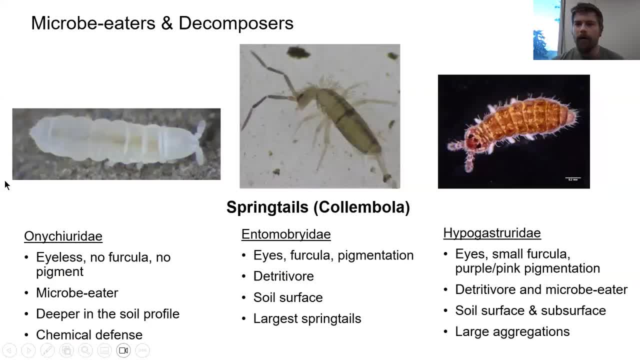 Sorry, They're a little bit bigger, Going back too fast. So the last group I want to talk about here are the hypogasturids. These guys are kind of in between the entomobreeds and the onychurids in terms of where they're living in the soil profile. 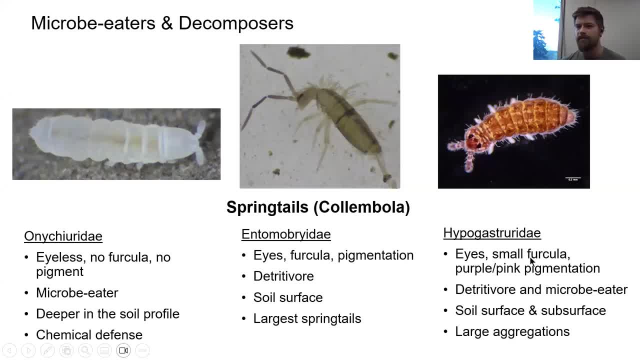 They have eyes, They have some pigmentation, But they have a pretty small furcula because they're not really using it to jump around too much, compared to say, like the entomobreeds. These guys again are detritivores and microbeeters, breaking down that litter on the soil surface, incorporating it back into the soil. 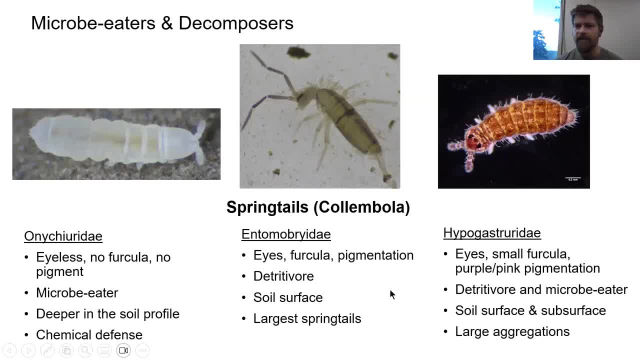 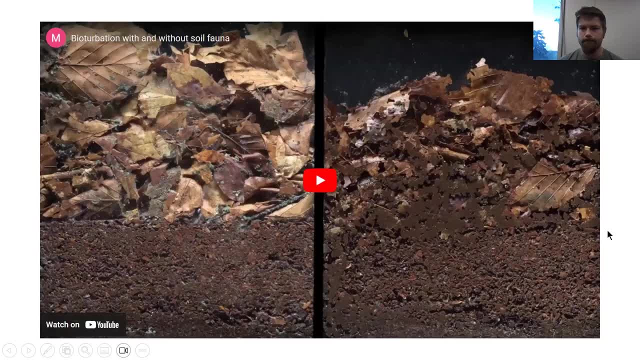 And encouraging nutrient cycling. These guys can actually often be found in really large aggregations too. All right, So we talked a lot about leaf litter, breakdown decomposers, And I just want to give you an example of really how important arthropods are to the decomposition process. Microbes are really responsible for, you know, ultimately carrying out these biogeochemical transformations. But microbes really- or, excuse me, arthropods- really make their job a lot easier and actually increase the rate of decomposition. So that's a reason why they're really important in our soil systems. 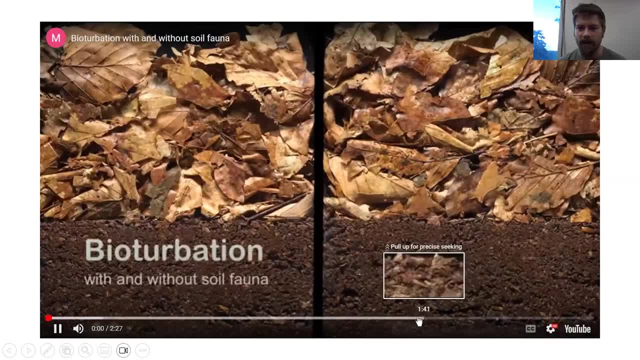 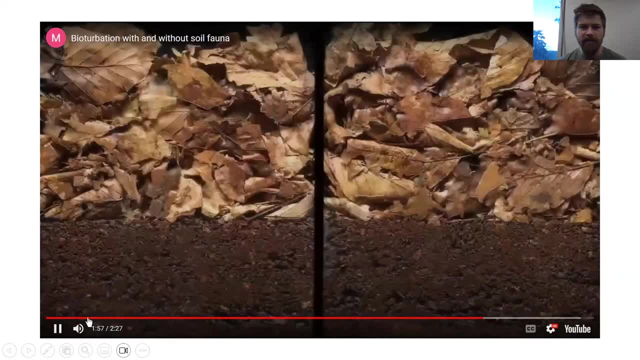 And I'm just going to share a video that basically shows that a lot better than I can say it, So I'm just going to fast forward up a little bit here, All right? So basically what we're looking at here is 15 weeks of decomposition in 20 seconds. 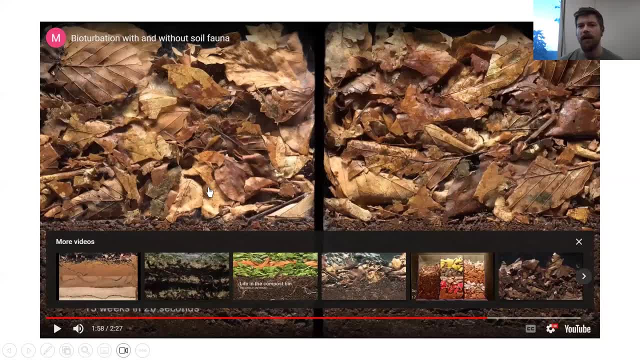 Wow, So that's a lot. And then on the left is decomposition in the absence of soil arthropods and other soil fauna, So just microbes. And the panel on the right is the decomposition in the presence of soil fauna as well as microbes. 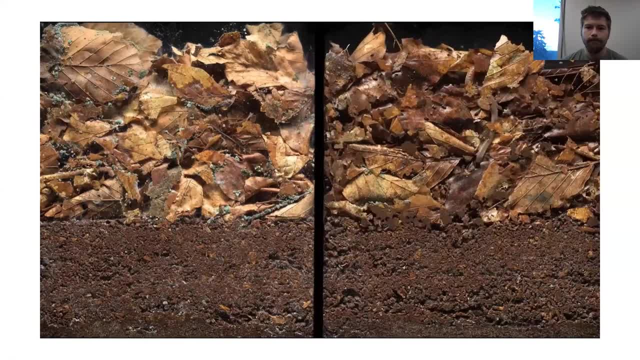 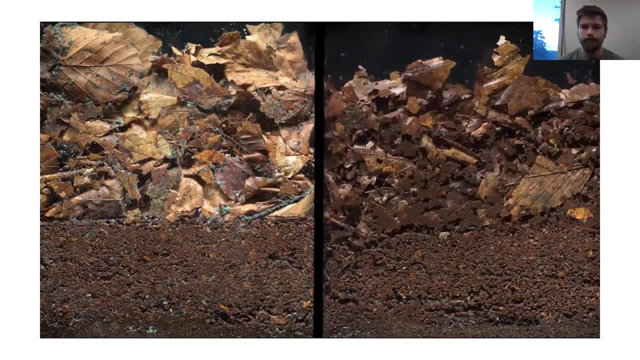 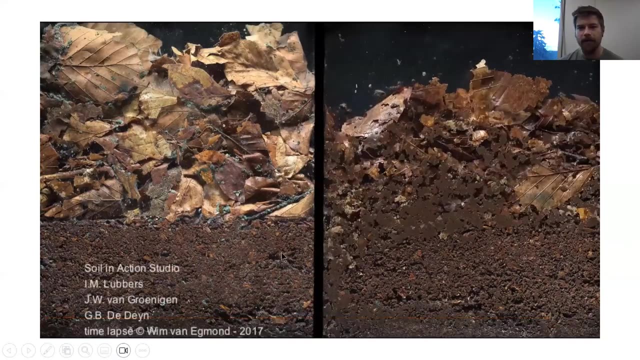 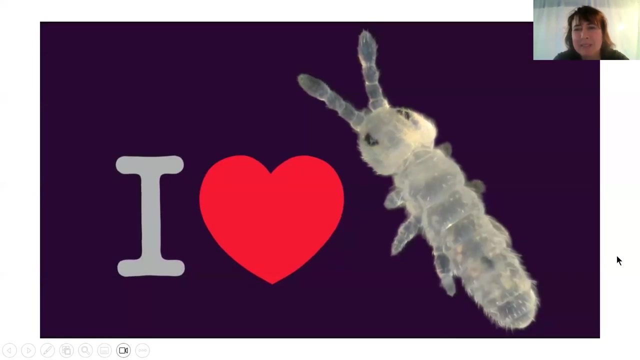 So just take a look And you can see that that increased rate of decomposition when arthropods are present in the system, You can see. you know things are starting to break down here on the left side, But really it's those, those columbula and those other arthropods that are really encouraging nutrient cycling and decomposition efficiency. 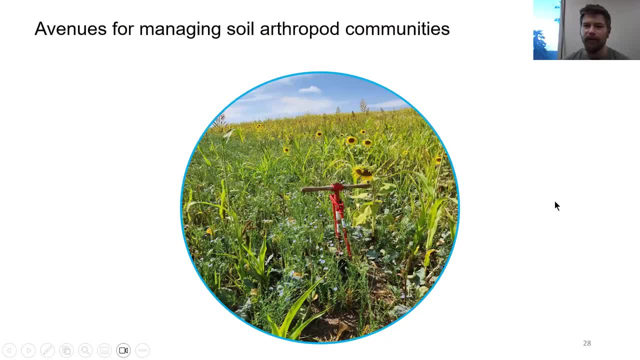 That's very impressive. Yeah, that's a really, really great video. I think it. Yeah, If you want to know why arthropods are important, in 15 seconds, That's really the video to watch. All right, So now I'm going to kind of shift gears a little bit here and talk a little bit just about some of the research that we've been conducting here and different avenues that growers, producers, people can take for managing soil arthropod communities. 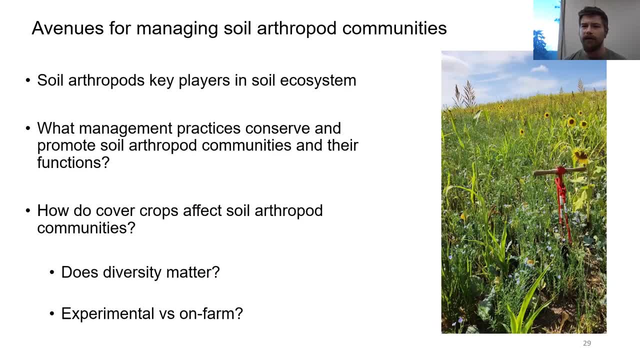 So, as I hope, I've convinced you guys that soil arthropods, through all these different functional groups, are really key players in the soil ecosystem, And so one thing that you know, we've been asking and we're interested in, in investigating, is: you know what, what types of agricultural management practices can conserve and promote soil arthropod communities, as well as their functions, just like we saw in that video. 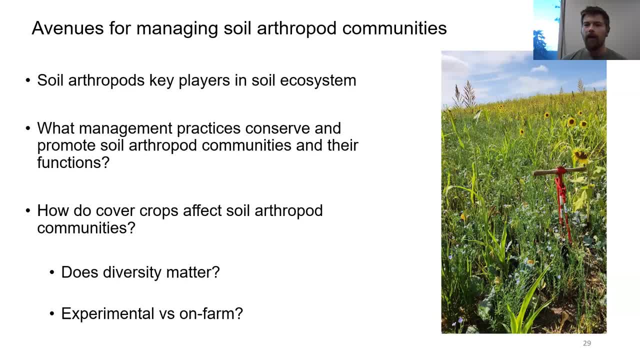 That decomposition video. And one thing that's you know people are getting interested in, producers are getting interested in here on the police: are cover crops Using cover crops as a way to suppress weeds? Yeah, So we wanted to ask: well, okay, so people are starting to use cover crops, how do those cover crops affect soil arthropod communities? and we kind of approach this a couple different ways. 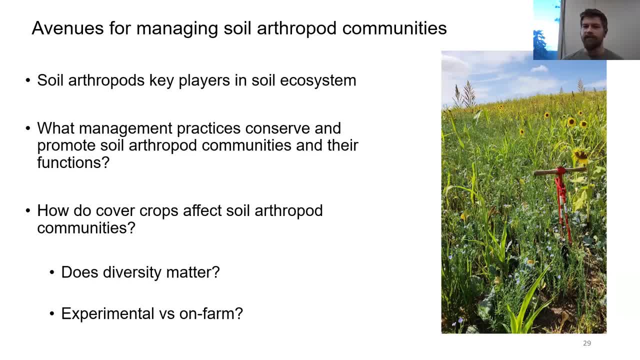 We asked: you know if people are using cover crops well. does the diversity of this cover crops matter? is a more diverse group, more diverse mix of cover crops better than, say, a model culture, and how does that impact our soil arthropod communities? 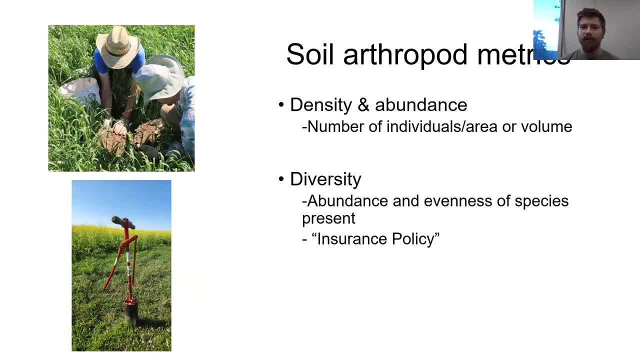 So I'm going to talk a little bit about a couple of soil arthropod metrics that we use to measure how different cover, crops and practices affect the soil communities. One of them is density and abundance, and this is really just the number of individuals per area or volume. In our case, we're talking about the number of individuals. in 2000 are, excuse me, two liters of soil. 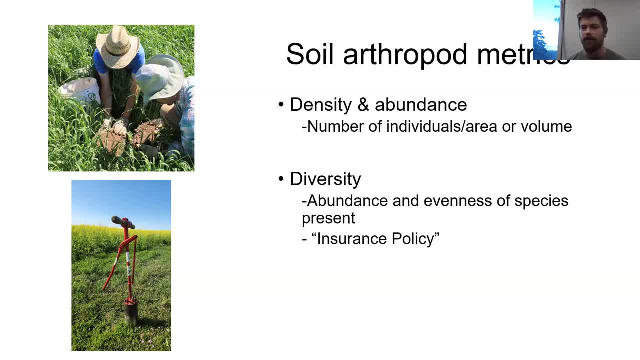 That's the. that's the size of the samples that we would go out and take and extract our communities from. That's the size of the samples that we would go out and take and extract our communities from. The next metric I'm going to discuss here is diversity, and this, basically, is the abundance and the evenness of the different species that are present in a community. 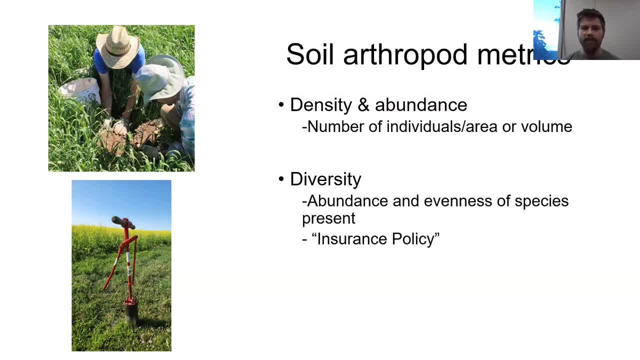 And I think diversity is a really important thing to think about and is, and is somewhat desirable from a ecosystem service perspective. because if it, If you have a diverse group of soil arthropods that are accomplishing all these different policies, Right, If you have a diverse group of soil arthropods that are accomplishing all these different policies. 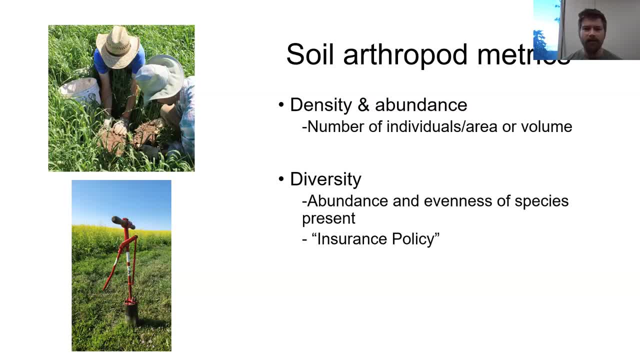 If there is, you know, some type of management practice or you know environmental events that that takes out one group that's doing a certain function, Do you have a diverse group of our diverse community of soil arthropods? there's another arthropod that's ready to step up and fill in that role? 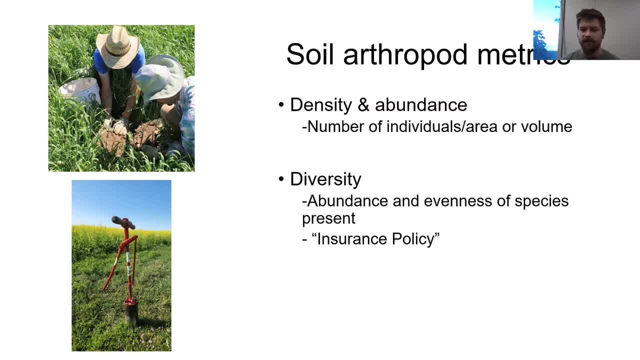 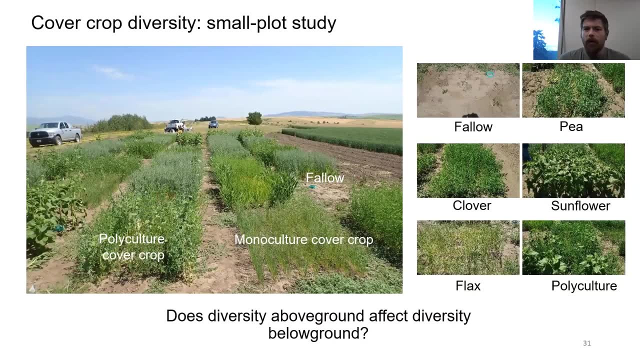 Again providing this kind of resiliency to the ecosystem. All right, so let's talk about cover crop diversity. So we were interested in understanding how diversity above ground, in terms of cover crops, affects diversity below, And so, to get at this question, we set up a small plot study in Pullman looking at six different cover crop treatments: fallow control, where we just didn't grow anything. 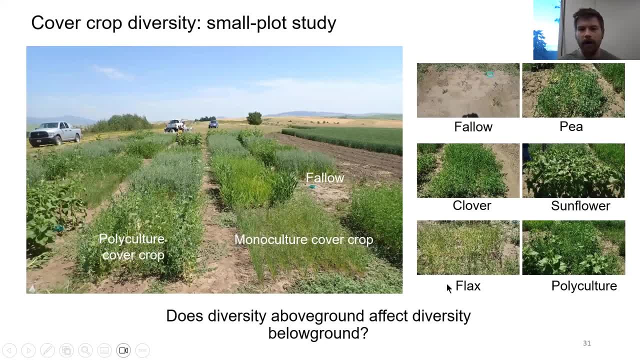 P clover, sunflower and flax monoculture cover crops, as well as a poly culture or a four species mix above ground, All of these different monocultures, again asking the question: does the diversity of cover crops above ground effect? diversity below? 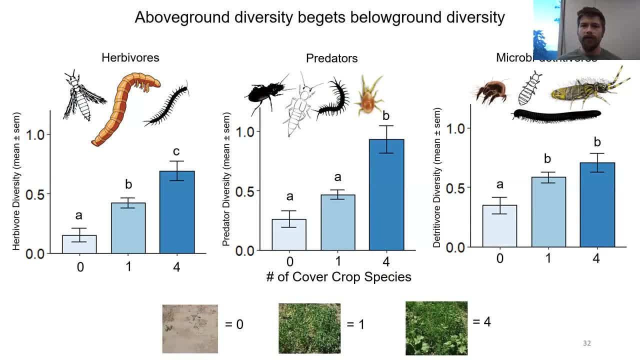 And here are some of these results. So, long story short, we did see a trend in above ground diversity, increasing the below ground diversity of all these three different functional groups that we just discussed. However, when we start to look at these data a little bit closer, 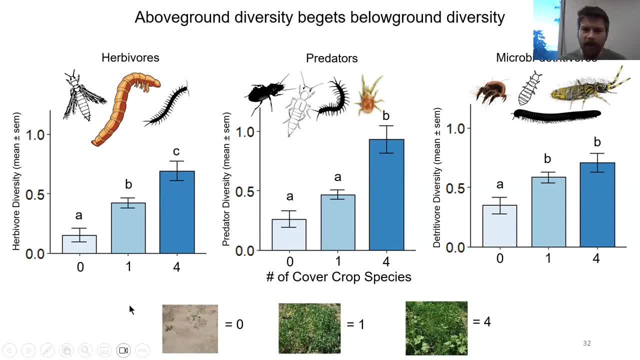 I think some kind of interesting patterns start to emerge. So just to kind of orient ourselves here quick, We're looking at this. this y axis here is going to be the diversity of our different functional groups. in this case, here we're looking at herbivores, predators, and these micro, micro beaters and decomposers, and then on the 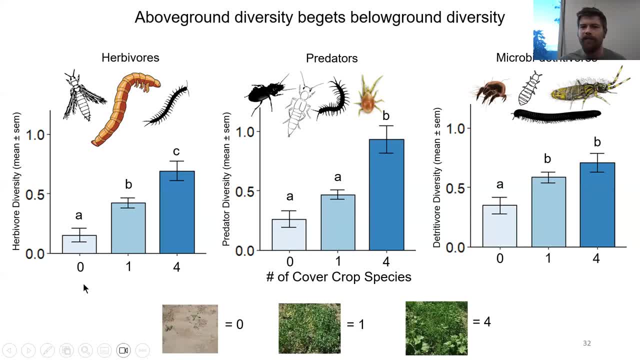 x axis. here we're looking at the number of different species in our cover crops. so zero is the fallow. The one is all of those model cultures and the four, And so we're looking at all of those monocultures and the four. 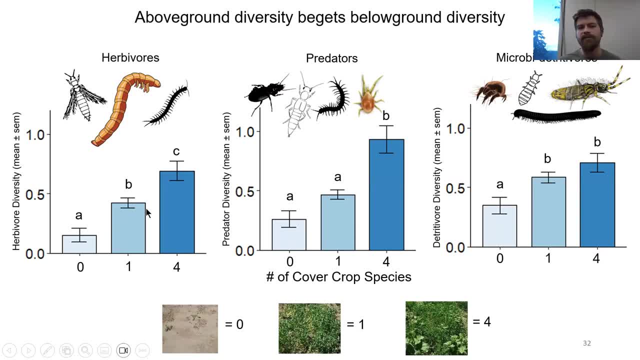 is this polyculture mix, and again we see this kind of increasing trend moving from zero to four in terms of promoting the biodiversity of soil, arthropod communities. but when we take a closer look at these data like, for example, our predator groups, we actually don't see any significant. 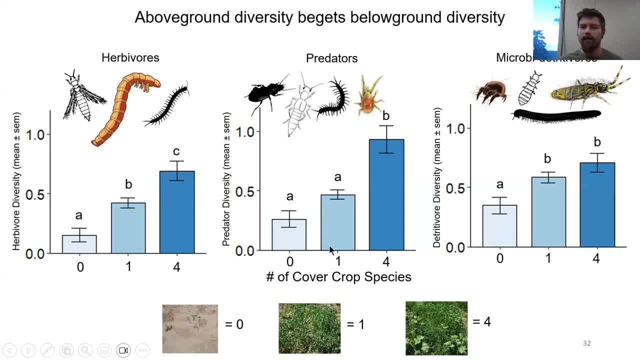 benefit moving from zero to one species of cover crops in terms of the effects of the biodiversity of our predator functional groups. you really need that multi-species polyculture cover crop to see a significant increase in predator biodiversity. when we look at our micro beaters, 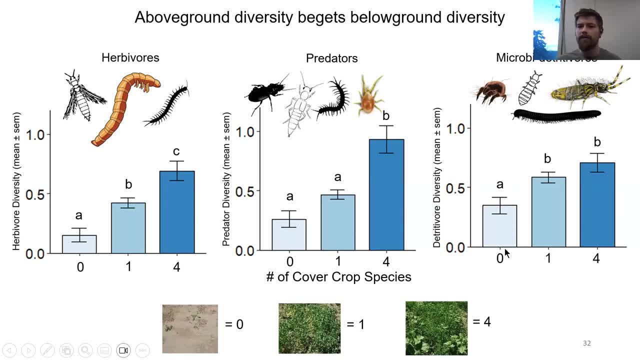 and decomposers. on the other hand, just moving from zero to one monoculture or, excuse me, zero to one cover crop, you do see an appreciable increase in this decomposer diversity, whereas moving from one to four cover crop species, you actually don't see this significant. 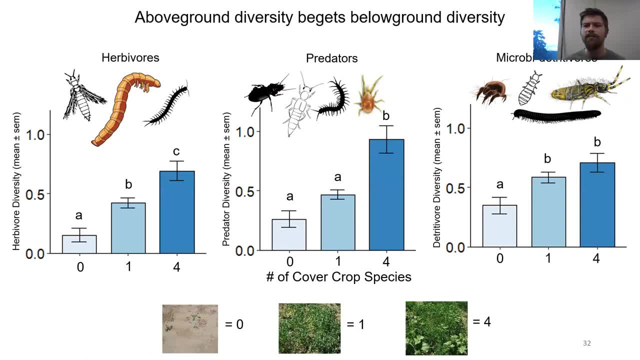 increase in in biodiversity, and so i like to point this out, just because it's a way of you know, thinking about how people can- or producers, people can potentially ecologically engineer their agro ecosystems to support below ground arthropod communities that have maybe desired functions like, for example, predators and their ability for biocontrol. 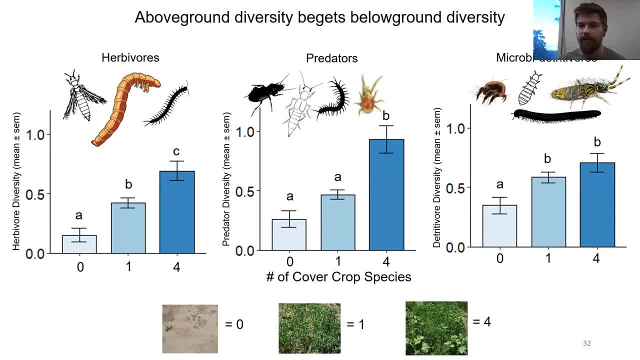 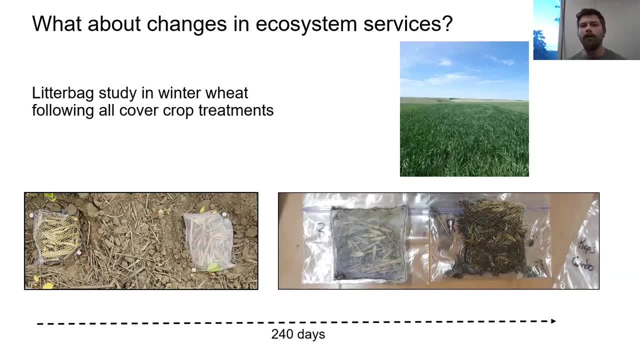 or these micro beaters and decomposers and their ability to enhance nutrient cycling. so one thing that we, you know, always like to to, to ask after we see a you know shift in biodiversity or community composition is like: what about changes in ecosystem services? so are these. 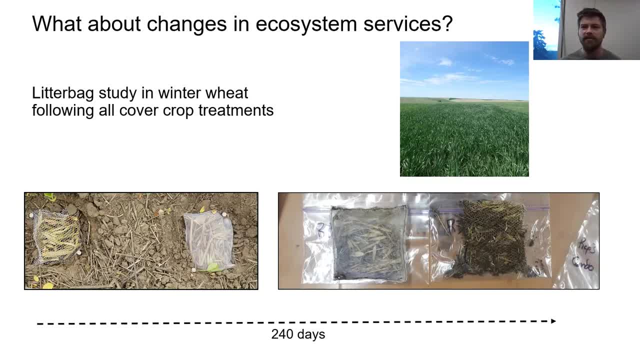 changes in biodiversity actually translating into changes in function, and we wanted to address this using a litter bag study looking at how the potential for arthropod mediated decomposition changes in biodiversity. so i kind of want to jump in a little bit more and then i'll let you talk about how we can. 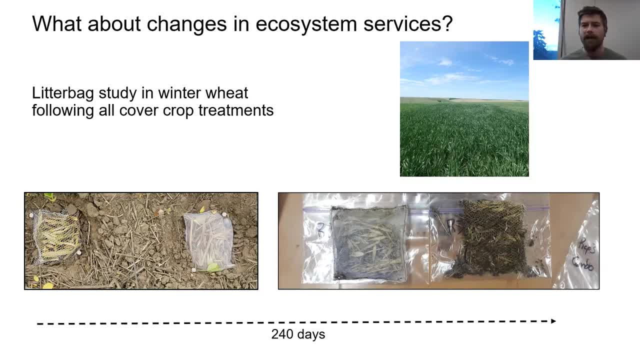 better understand this. this is a really interesting work in using of thinkers with interest in this, in the juxtaposition you know, looking at the different subgroups of a business that are selling rice seedlings in the iowa bay, and then on and on. for the past few weeks, 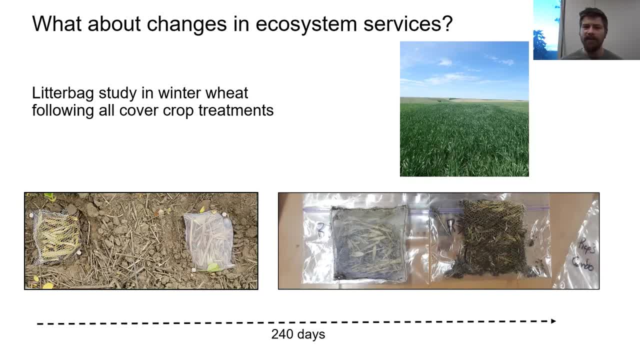 we then started looking at how to, uh think about how we could manage a natural heritage. 맞아요, we actually found a method where we, you know, did a system services, in this case, decomposition of the soil, arthropod communities, And so this litter. 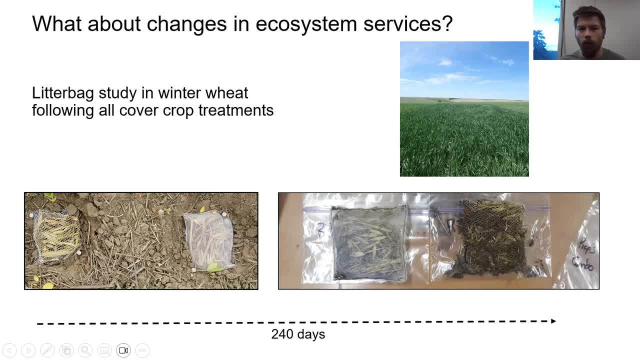 bag study. we had two different mesh sizes right, One that allowed arthropods to enter and access the litter and one that excluded them. So you can kind of think back to that video that we just saw. It's basically the left and the right panels. So we set that out for 240 days and then we recovered. 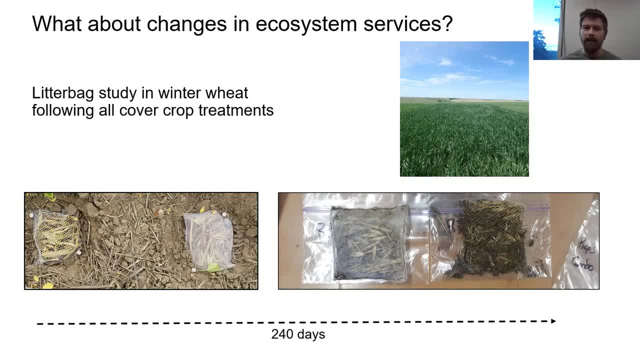 them And we calculated the litter decay rate for each of these bags in winter wheat following those cover crop treatments. And you can already see, looking at these bags right, It kind of resembles the video that we just watched here. Like with this bag is the bag that had arthropods. 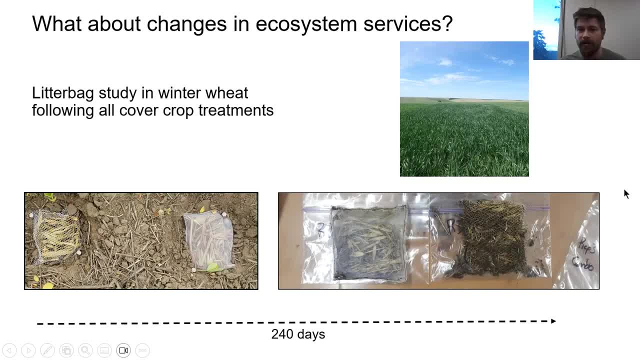 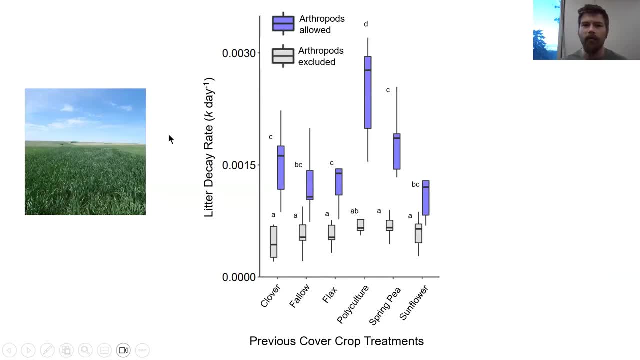 allowed to access the litter, whereas this bag excluded arthropods from accessing the litter. All right, So here we're looking at again the litter. So this is the litter decay rate of litter in winter wheat following all of our different cover crop. 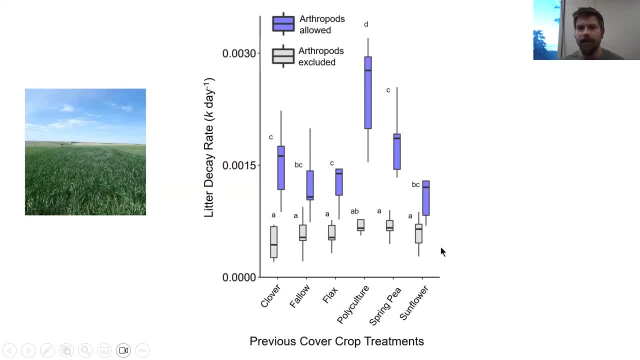 treatments And we've got two different boxes here. The white boxes are the litter decay rate when arthropods are excluded And the blue boxes are the litter decay rate when arthropods are allowed. So right away we can see that when arthropods are allowed to access the litter. 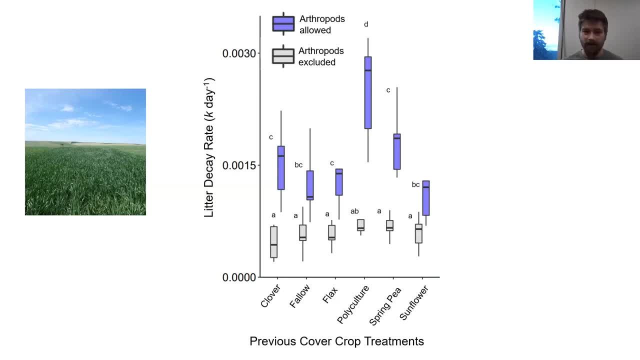 there is a significant increase in litter decay rate. We didn't really see any differences between litter decay rate when arthropods were not allowed to access the litter. However, when we take a look at the decay rate in the bags that arthropods were allowed to access, 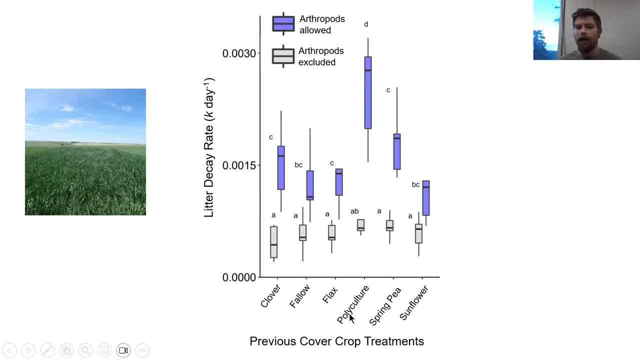 we kind of see an interesting pattern here developing when there is an increase in litter decay in the polyculture or the multi-species cover crop treatment or, excuse me, in the winter wheat. So we can see that there's an increase in litter decay in the polyculture or the multi-species cover crop treatment or, excuse me, in the winter wheat. 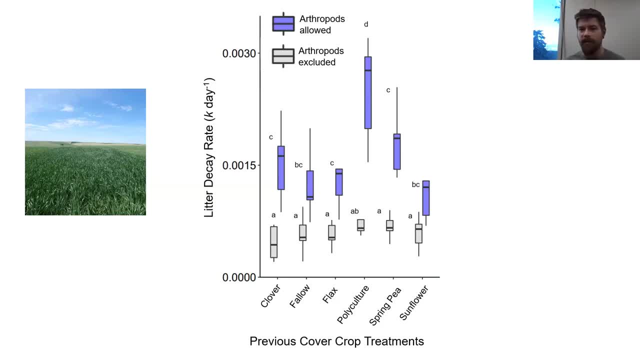 So we can see that there's an increase in litter decay in the polyculture or the multi-species cover crop treatment or, excuse me, in the winter wheat, following the multi-species cover crop treatment, compared to the other monoculture treatments and fallow. 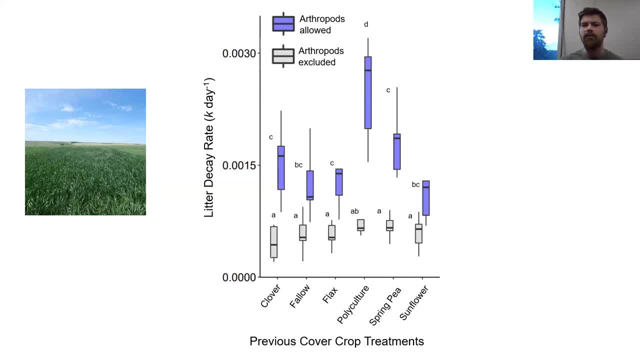 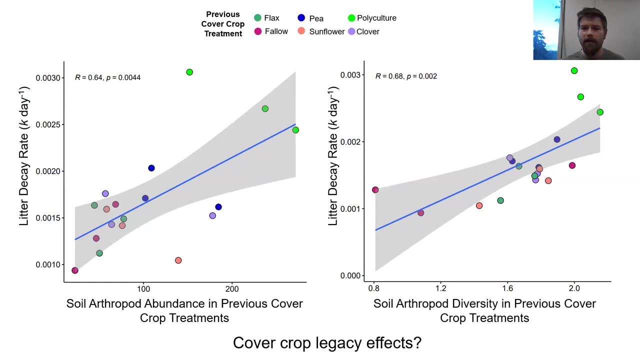 So, again, you know, this is kind of indicating that, you know, perhaps this increase in biodiversity promoted by the multi-species cover crop is translating into an effect on ecosystem services. And indeed when we, when we look at you know, the litter decay rate again here on the Y axis and our soil, 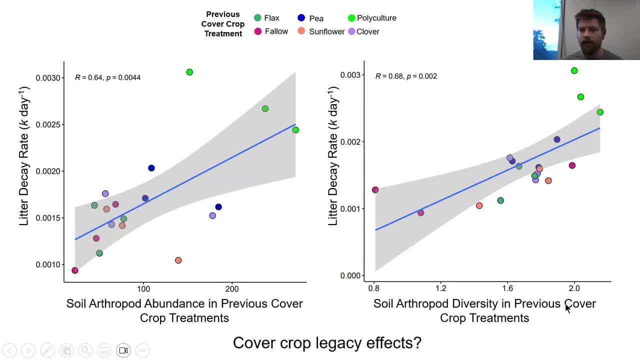 arthropod abundance in the previous cover crop treatments and the soil arthropod diversity in the previous cover crop treatments, we're seeing a very positive correlation between litter decay rate and both abundance and diversity in the previous cover crop treatments. And when you look at the specifics here, for example these green dots, this is the diversity in the polyculture treatment and this is the abundance in the polyculture treatment. 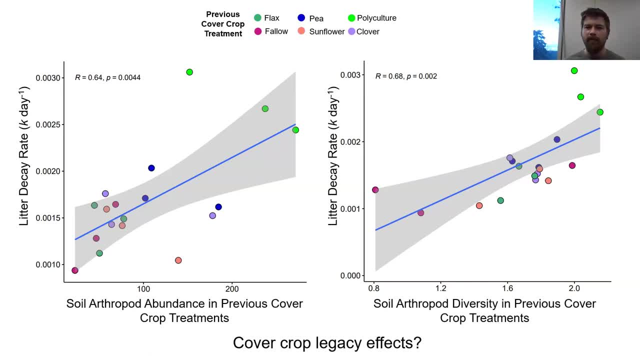 So you know, again it's suggesting that there's potentially some cover crop legacy effects that are happening. That's again promoting this arthropod mediated decomposition in the cash crop following these different cover crops. So I would say that's a pretty positive thing from a agronomic standpoint and is especially important for folks out there that are using no-till or conservation till practices. 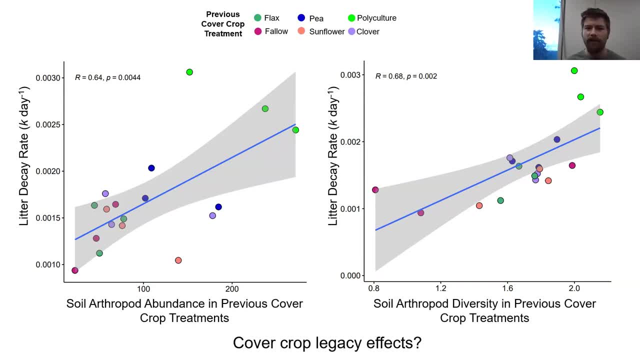 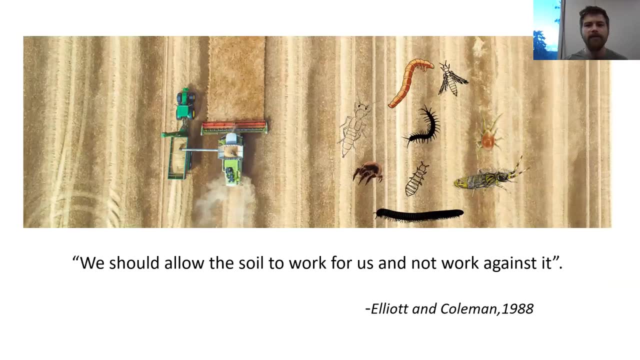 because you really do need some way to to reincorporate that litter into the soil, and arthropods are going to be a big part of that practice. So I just want to return here at the end of the presentation To this quote that we kind of started out with. you know what is soil health? 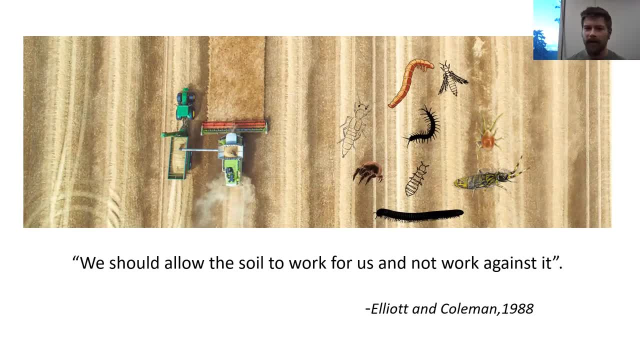 Well, it's this idea that we should allow the soil to work for us and not work against us- excuse me, not work against it. So practices like cover cropping that can promote these arthropod communities and their potential ecosystem services are are one way that I think we can help the soil work for us. 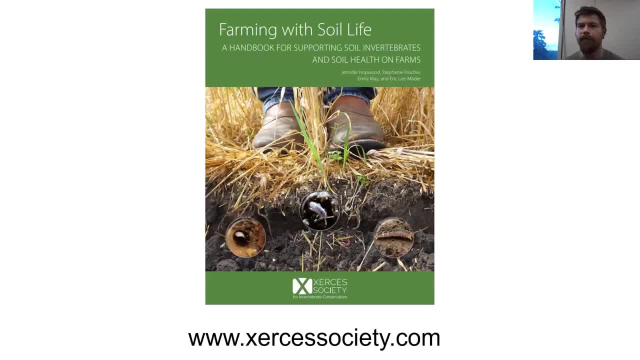 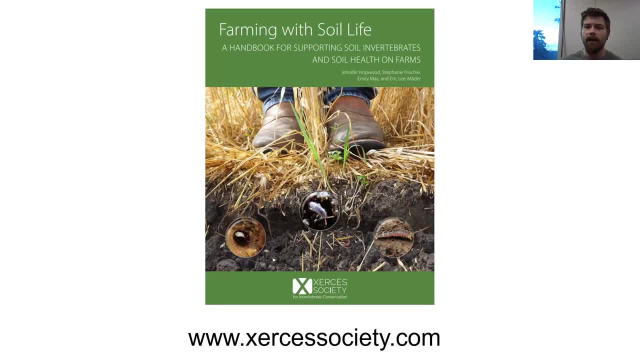 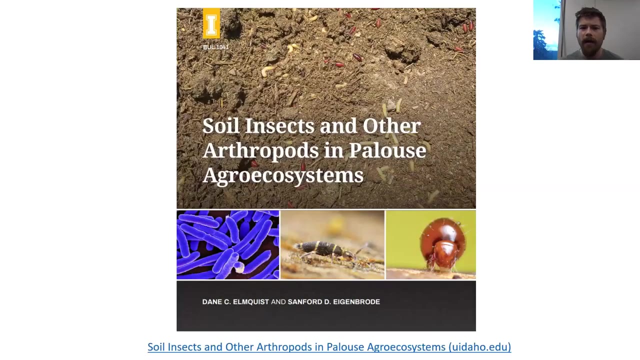 vertebrate conservation called Farming with Soil Life. It's, you know, hundreds of pages of great pictures, great management recommendations and a lot more information on soil biology than we can cover here today. So that's a great resource I'd encourage you to check out. And then Stanford and 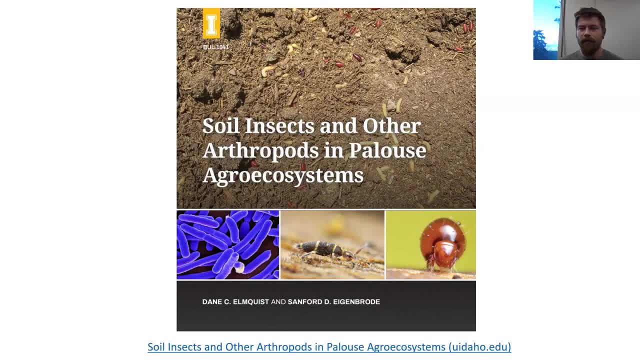 myself. we just published this bulletin through Idaho Extension called Soil Insects and Other Arthropods and Palouse Agri-Ecosystems, which is a basically, you know, a shortened version of this talk that we just went through, So that's again available for free download on the University of 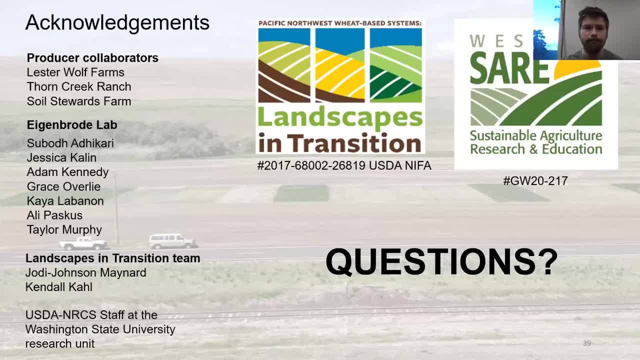 Idaho Extension website and I'd encourage you to check that out. Just I'd like to acknowledge our funding sources that supported this work, as well as our great team here at the University of Idaho, and I'd be happy to take any questions. Thank you, guys, for your time. 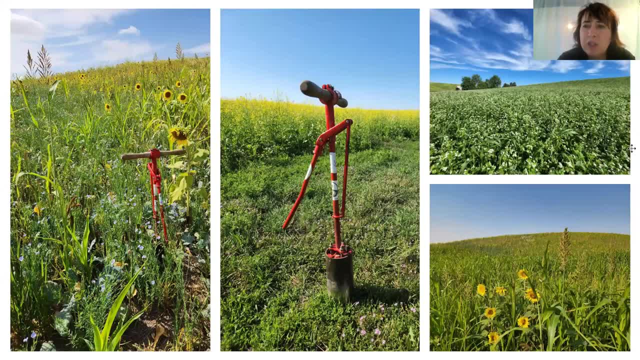 Yeah, Thank you. If there are any questions, just feel free to shout them out, or I have a couple in a second. But first of all I'd like to say that's a beautiful presentation. I really enjoyed watching your or looking at all your graphics and stuff. That was really well done. 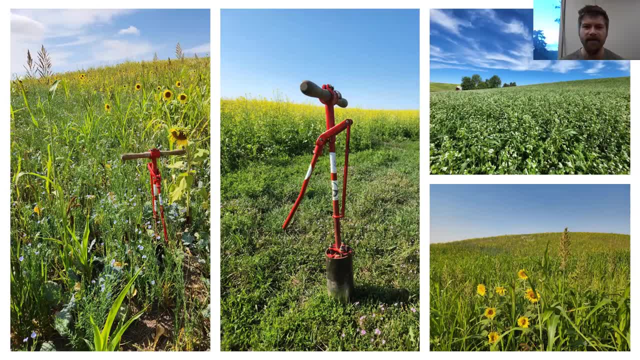 Yeah, thank you. It's nice to actually share, you know, photos of these guys, right, Because they live in the soil, so they really go unnoticed And so we have to. yeah, I feel like that's my job is. 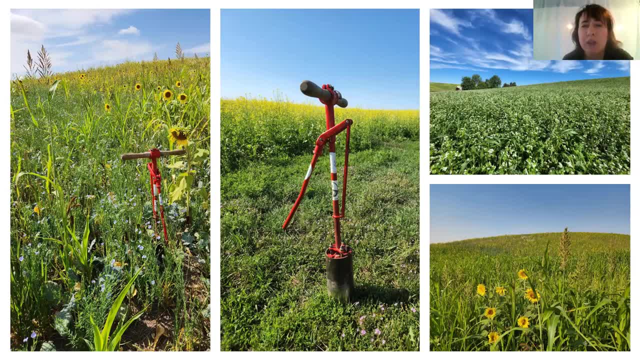 to help. Beautiful photography had some really beautiful pictures there of the insects I mean so much better than you see some sometimes. you see those guardian ones have just a blurry picture of a you know something you're like. I'm not really sure what that is, but it lives in the soil, So 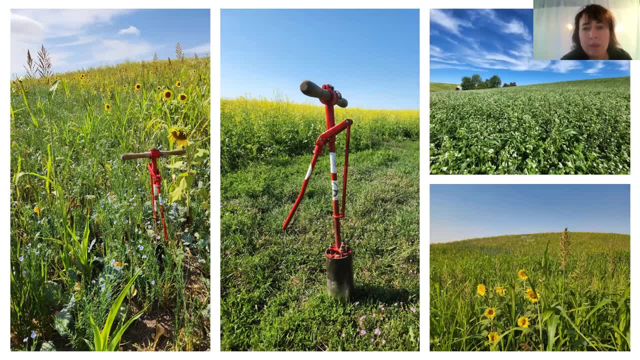 it's kind of nice to see the representation of that. Yeah, and there's that extension bulletin as well, as is packed with pictures too. So if that's up your alley, yeah, definitely, Yeah, I plan to check that out too. 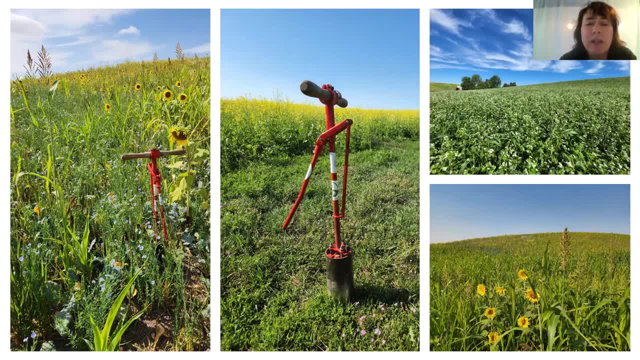 I did have a couple Questions about your experiment When you had the land follow. was it just that you just did it planted and allowed it to remain bare, Or do you have to have do anything to keep it bare? Yeah, great question. So yes, basically we just didn't plant anything, So there was no like. 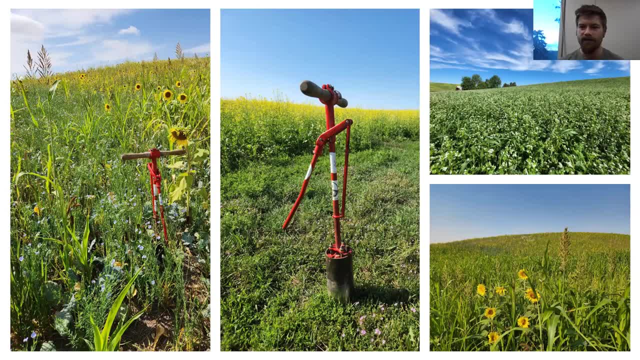 we didn't chem follow it or anything, no tillage, It was just just remained unplanted. So there were some volunteer weeds and stuff too that that didn't, you know, crop up In the in the fallow system. But yeah, just unplanted. 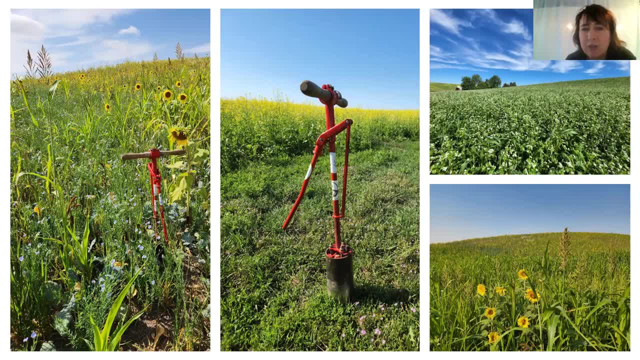 Did you have any questions there, Vern? I noticed that you turned off your mute. Well, I was just wondering what the effect of pesticides are on you know different pesticides are on the soil arthropods. Thanks for the question, Vern. Yeah, that's a. that's a really great question, Really important. 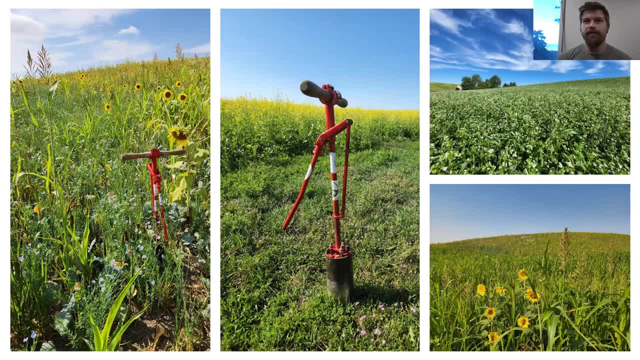 So the amount of research of pesticide effects on soil arthropods is nowhere near as much as we know about above ground. However, we do know that- and this isn't research from our lab. this is some data generated from other labs out there. One lab specifically looked at the effect of 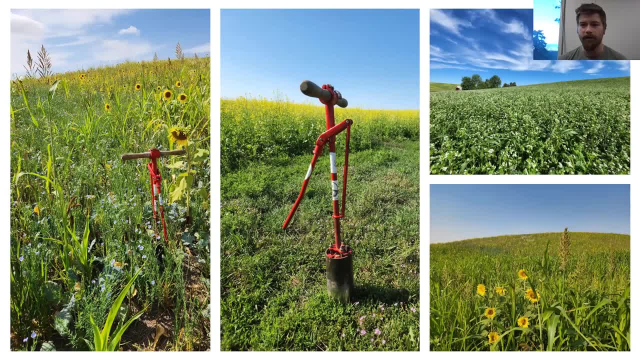 neonicotinoid seed treatments on decomposer- excuse me, decomposer soil arthropods and their ability to decompose litter using a litter bank study And they found that when arthropods were exposed to neonicotinoids, treated seeds that or in fields with neonicotinoid treated. 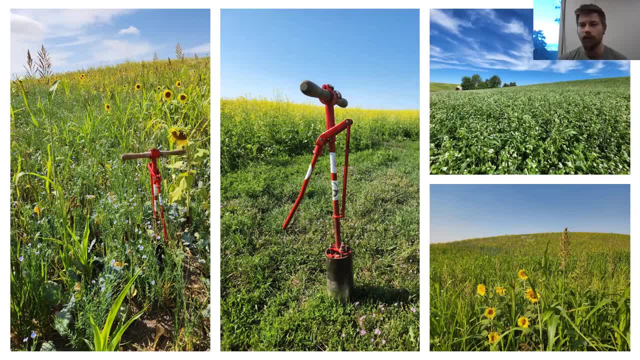 seeds, that the abundance of decomposers decreased, as well as their ability to actually break down the litter decrease. So there are some negative effects, at least with seed treatments on these groups that we know about In terms of like herbicides. I think that's one thing that's still. 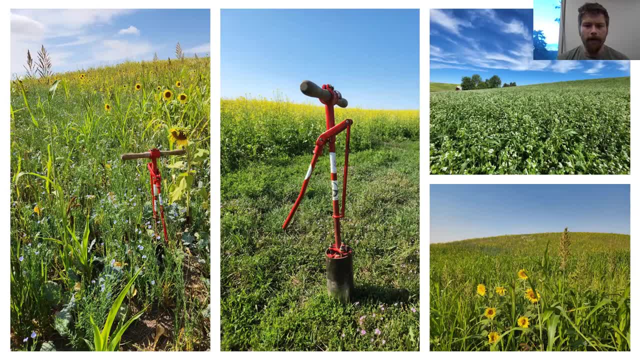 relatively unknown, at least for this region, And so that's definitely an area where we we could stand to learn more, more about the effects of herbicides, but certainly, certainly insecticides specifically, and and seed treated neonicotinoid seed treatments. 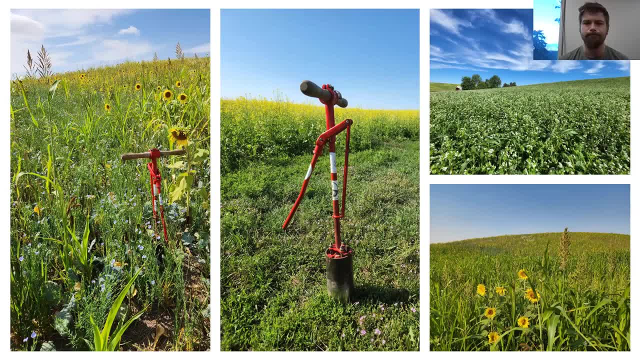 do have a a negative effect on these guys. I kind of figured that. Yeah. Yeah, That's one. one drawback of, you know maybe, prophylactically treating all of our seeds that's planted is, yeah, you might be losing out on, you know, potential for some of these. 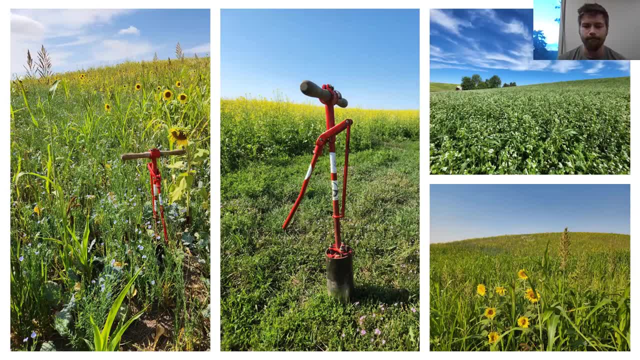 these free ecosystem services like decomposition? Yeah, Did. did you have any other questions? I don't think so. I enjoyed the program. Oh, I thought it was excellent. You did a. you do a very good job of presenting. It was very fascinating. 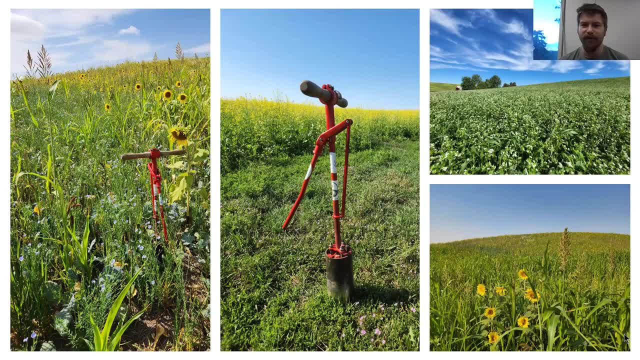 Happy to, happy to share, and you know, share the share, the world of soil anthropos with people. Again, I think this is one group that maybe goes underappreciated compared to, say, earthworms and you know, more recently, the, the soil microbiology. you know, with the advent of DNA sequencing and stuff, 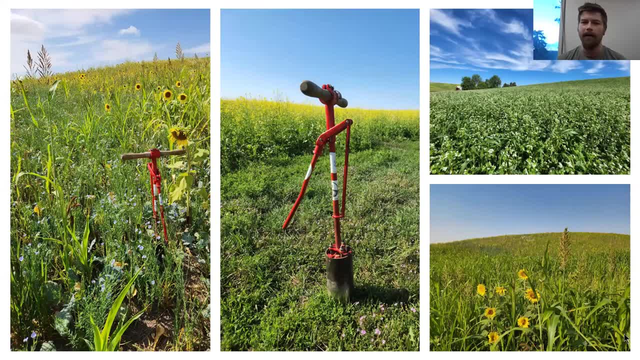 people really jumped on soil microbe training. Obviously they're super important, but I always, I always think of these guys as kind of that, that in between right You've got the soil microbes on the small side, the earthworms on the larger side, and then there's this soil. 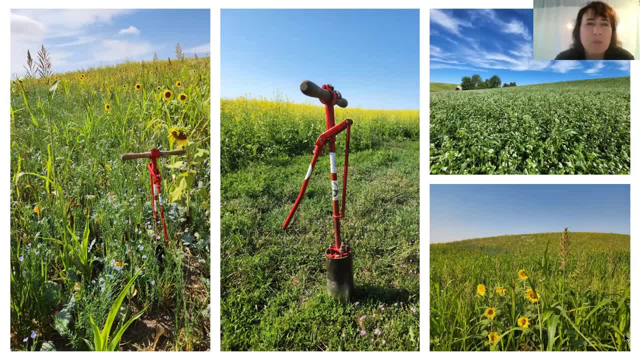 electrified group that fits in the middle. This is definitely a group that's underappreciated. I agree with you, Even when you know, like I said, I went through entomology masters and we did not cover this group near like we know now. I don't think it was studied. 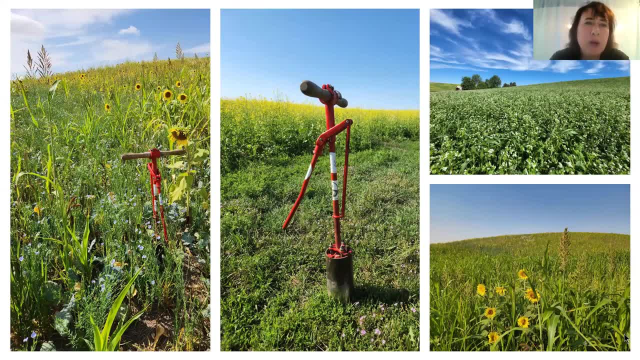 I did have one other question about the, the predators. I thought it was really interesting that the predators require a more complex ecosystem, kind of like they do above ground. Um, that was pretty fascinating. Yeah, Some similar, uh similarities there. 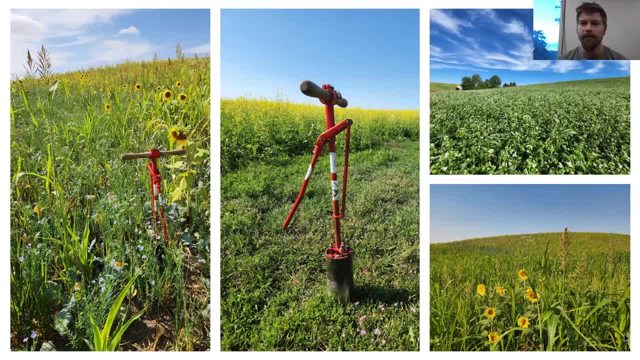 like you just alluded to, with the, with the above ground world, um, which is always something that's that's fun to, to find out. Um, yeah, I think that the, uh, the polyculture cover crop and the. 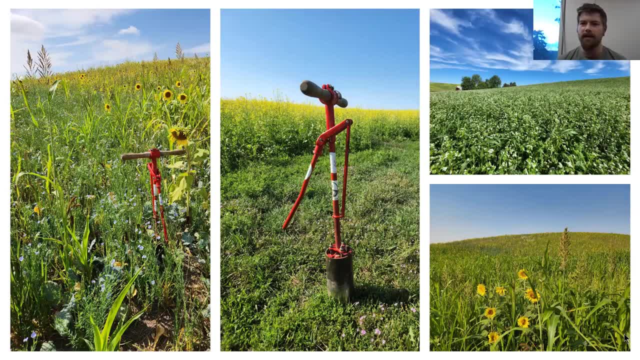 you know, um, different rooting systems probably provides um a little bit more of this habitat heterogeneity, um which is really really important for predators, Um, and so I think that you know just kind of speculating here. I think that might be one reason why we're seeing. 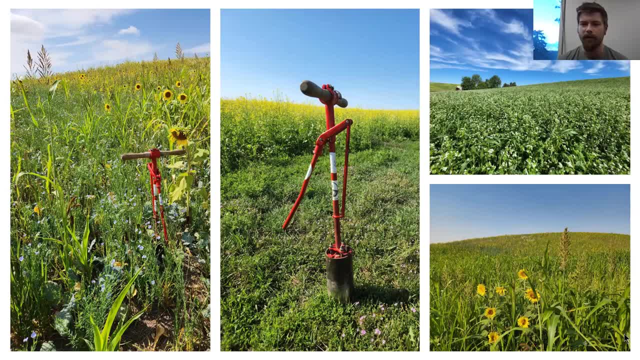 that that increase in their diversity is just gives them a little bit more of a heterogeneous habitat. Yeah, That's what I was wondering, just what you said, if you had any any different viewpoints as to different reasons why predators need more diversity. Yeah, I'd say that's.